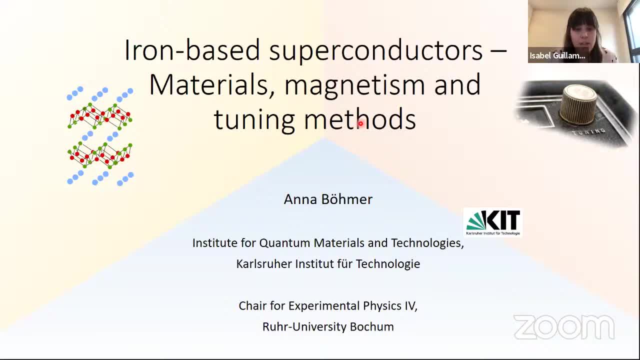 your hand and I will unmute your microphone so you can ask the question yourself. With this I'll finish. Thank you all for coming and, Anna, the stage is yours. Thank you, Isabel, for the nice introduction and also for the invitation to the seminar. It's a pleasure. 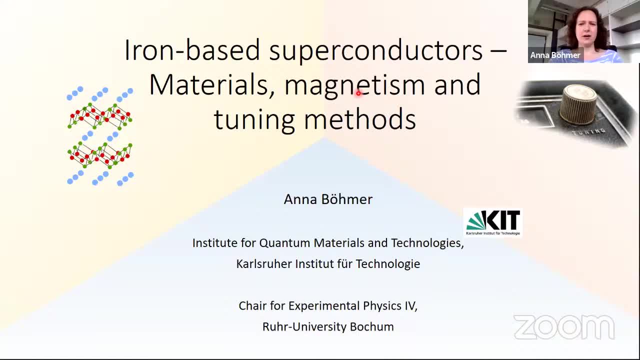 Thank you, Isabel, for the nice introduction and also for the invitation to the seminar. It is a pleasure, um i i thought i would show you a few uh interesting results on the material class that i've been working on for many years now on the rms superconductors. what kind of materials? 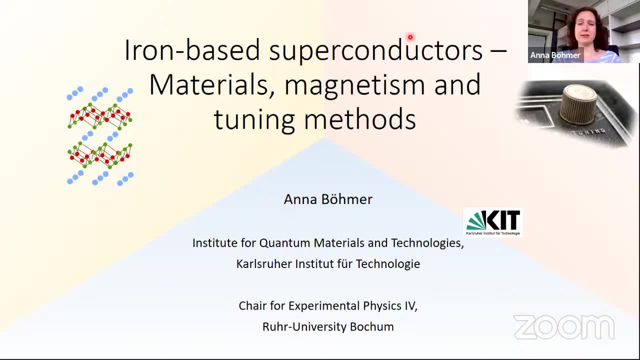 we're working on, then one of their interesting properties is their magnetism and we will see how these are interesting magnetic materials and tuning methods, how to change their properties, change their magnetism. tuning, i think, is a nice word. it really comes from the radio technology when you tune a frequency, so that's my symbol for tuning, but we use it frequently in this field to 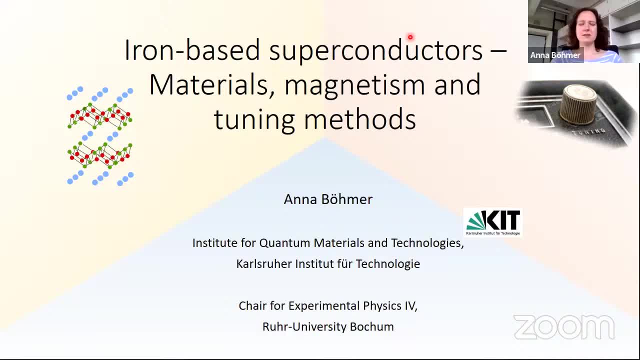 mean change material. um, as isabel said, i was, or i've been, at cultural institute of technology for quite some time. um, this is where most of this work has been done, and now i'm at the chair for experimental physics four in bochum. so basically here. 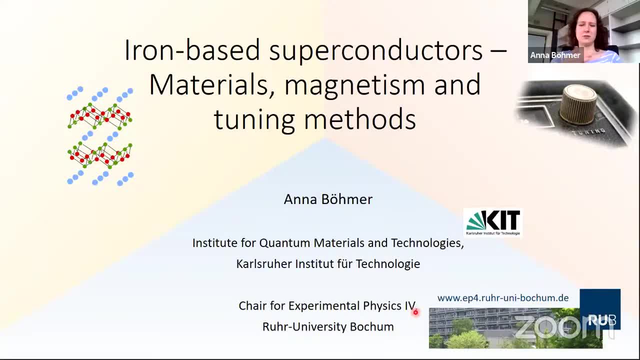 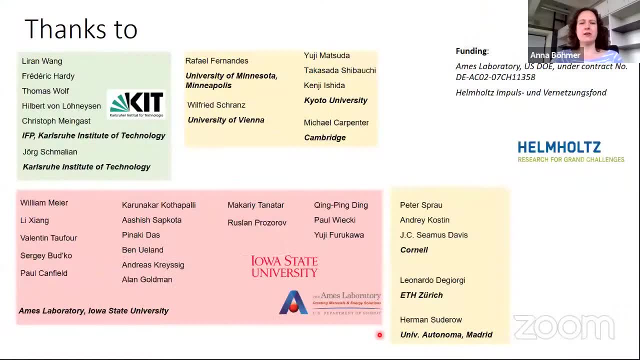 experimental physics forest. well, there's, uh is the name of the institute. it's also on the fourth floor. um, this work has not been done alone, and here i list collaborators. there's a large group at the cultural institute of technology. there's another large group where i did my postdoc at the 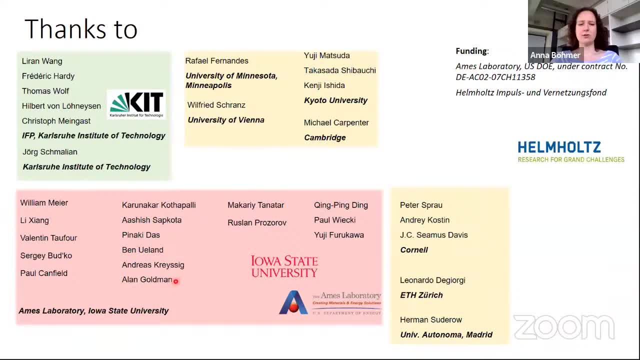 ames lab and the paul canfield's group. there's also the scattering group there and goldman is the leader uh nmr group, another low temperature group, and external collaboration collaborators all over the world, be it in the us, in vienna, in kyoto, in zurich and also. 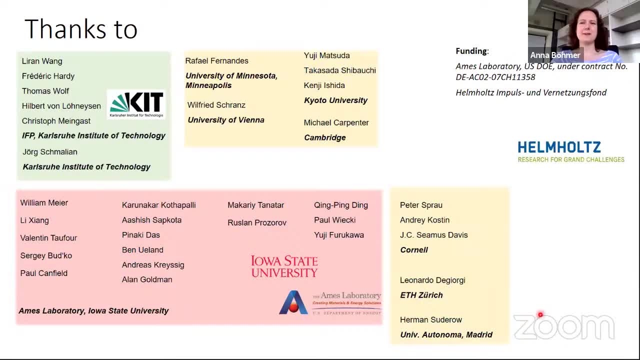 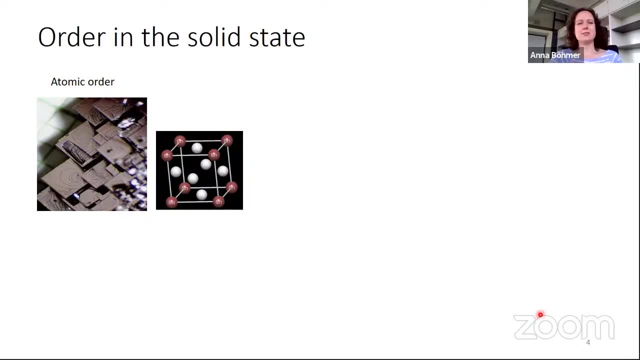 were had some very nice workers, herman, i'll mention it as well. so let's start general. what do we study? what one thing we really like to study is order, order in general terms. if we look at the crystal, at the material, the crystalline material, what we have is atomic order, the atoms or the ions. 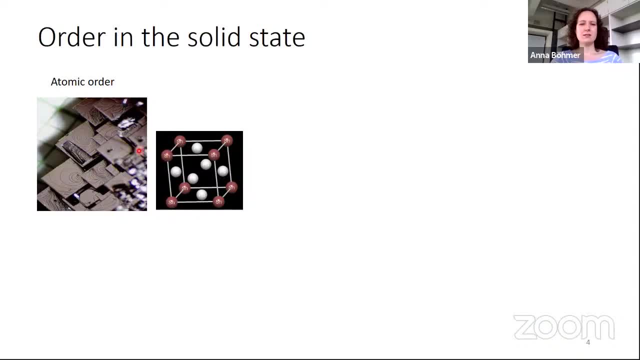 are in specific places and because in this case the atoms are arranged in this cube structure. the crystal looks like little cubes, so we can really see it. this is a millimeter scale. we can see how the atoms are arranged there. there are other kinds of order, and one of them is: 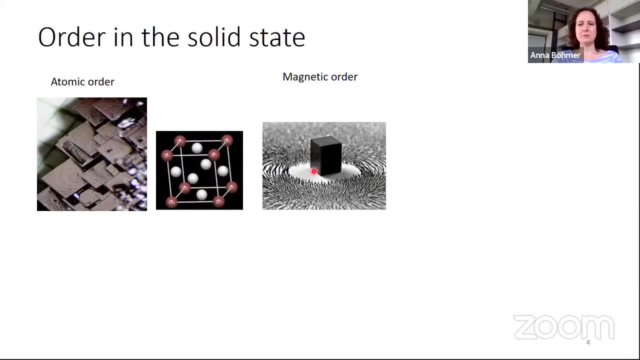 magnetic order, that's your fridge magnet, for example. what we have here is the spins on the sides of these electrons. they are ordered, they say, in the fridge magnet. all points in the same direction. but there could be other kinds of magnetic order. one famous one is antiferromagnet, where they are alternating up and down, up and down, but in an auric fashion. 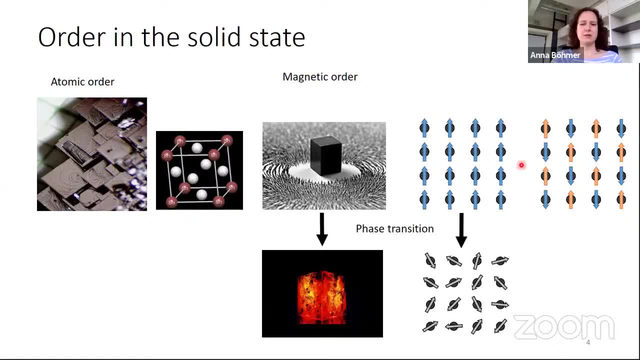 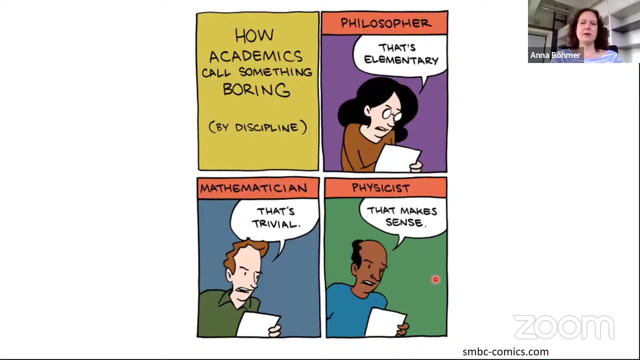 what happens if we destroy order? we know that from daily experience. we can melt a crystal, we can also heat up the fridge magnet. at some point it will lose magnetic order. the spins will be disordered from like thermal excitations. that's a phase transition and well, that's something we understand and i really like to show this graph. 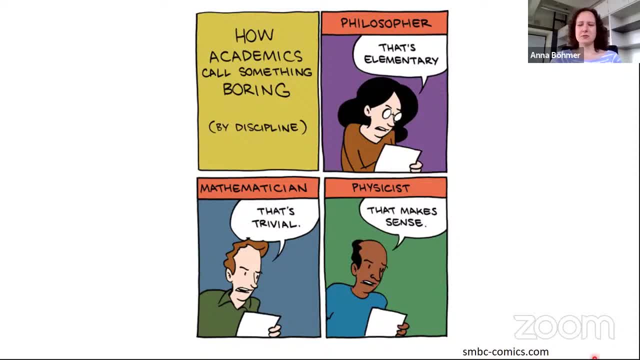 it, i think, tells us something about physicists. it's from saturday morning breakfast cereal comics- a nice site. it's how academics call something boring by discipline. so philosophers, that's elementary. when they find see something that's elementary, that's boring. mathematicians that's trivial. and physicists what they say is: that makes sense. 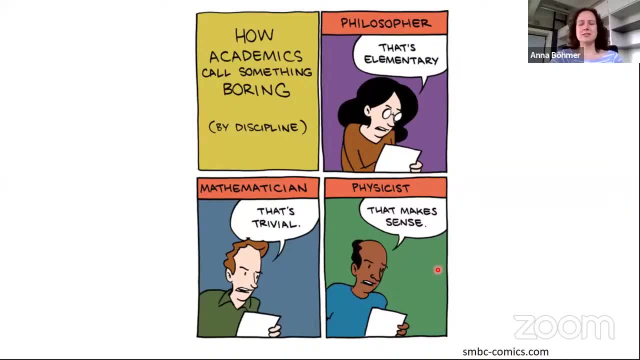 well, you see that physicists use plain language, but you also see, or what our understanding is, what we understand. that's boring. we want to find new physics, new materials, new phases, also beyond standard model particle physics. that's what excites us, and let's look at one of these things that we don't quite understand yet. 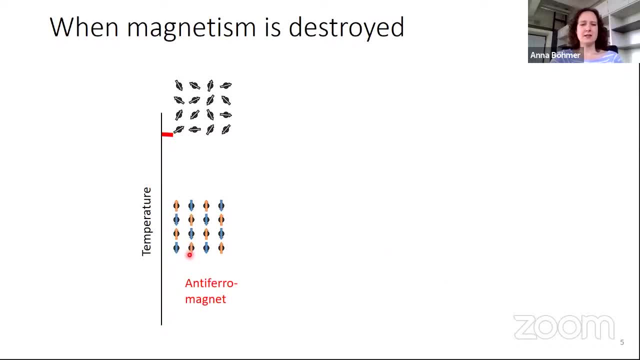 that is when magnetism is destroyed. we just had that. if you increase temperature, say, then you go from an ordered magnet to a disordered phase. but what happens if you change some other parameter, say pressure on a material or chemical composition, then this temperature will destroy the magnetism. 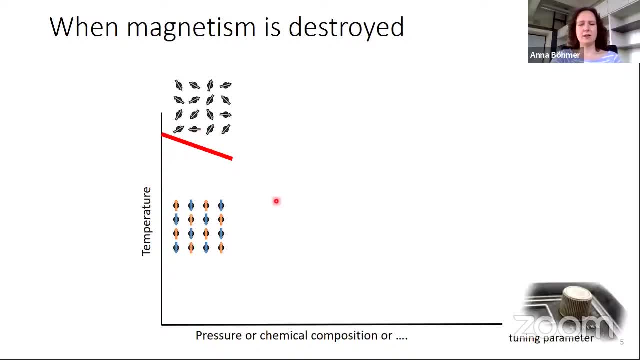 can change, can decrease, and it can, and this, this thing that you change, that's an example of tuning parameter. so we tune the phase transition temperature here, we can tune it further and we can tune to zero, and when we do that, what we find on the other side? well, you, typically 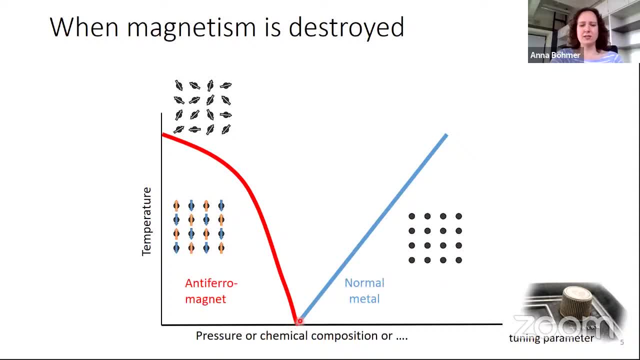 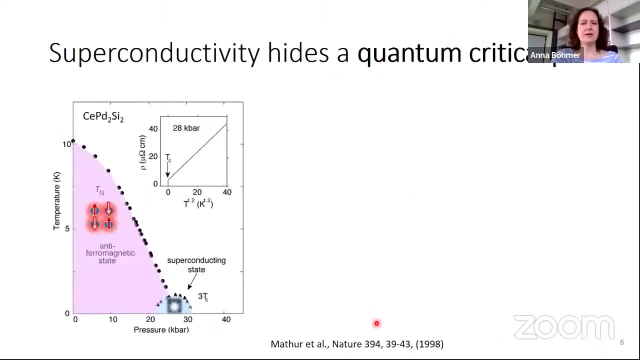 find normal metal, and the point that's interesting is here. here, the material doesn't really know what it should be. it should be a magnet, should it be not, and usually decides to do something else completely. here's where new phases can emerge, and one of these could be, or is, super connectivity. 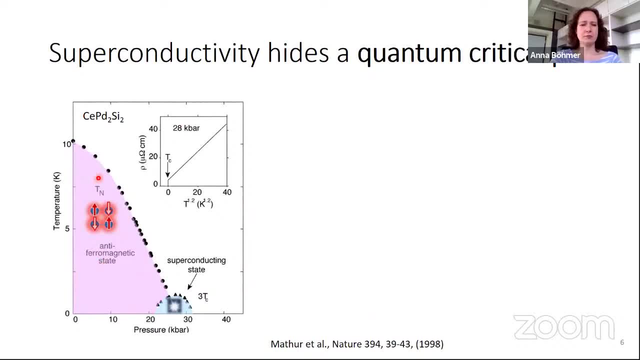 and this is one of the first cases where such behavior was observed. what we see here is an antiferromagnet serum relating to silicon tube and if you apply pressure to it- physical pressure- then this transition temperature gets pressed, temperature gets suppressed, just as we said, and we see a dome of a new phase, and this phase is a super connecting phase. 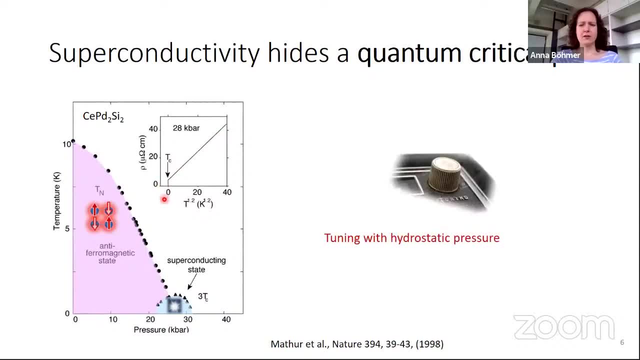 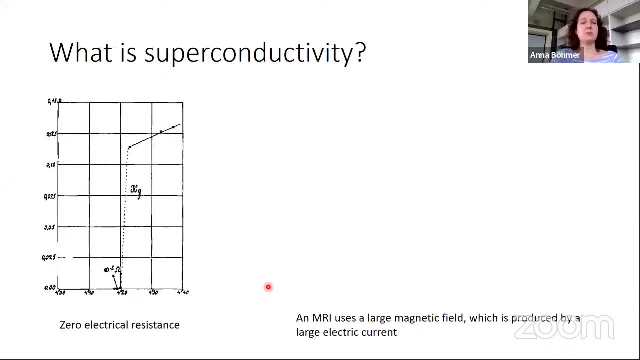 this is the electrical resistance: it goes to zero. so here we're, tuning with hydrostatic pressure, and now i want to tell you a little bit about what is superconductivity. superconductivity was discovered in 1911, so more than 100 years ago, and this is the original data. 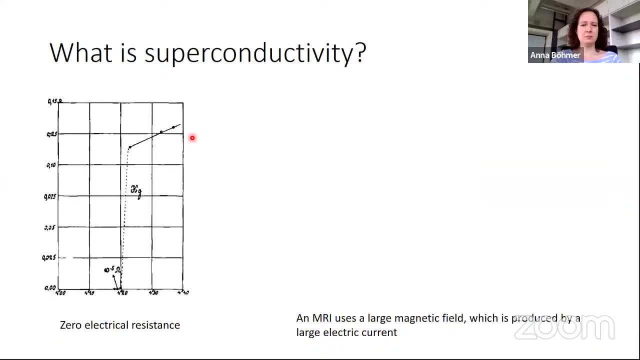 from heike kamerlingh: honest electrical resistance of mercury which, on cooling below 4 kelvin, drops from some finite value to exactly zero, or two, immeasurably small in his case, but it's zero. that's the point. so super connectivity, this is used nowadays. it's used, for example, in magnetic. 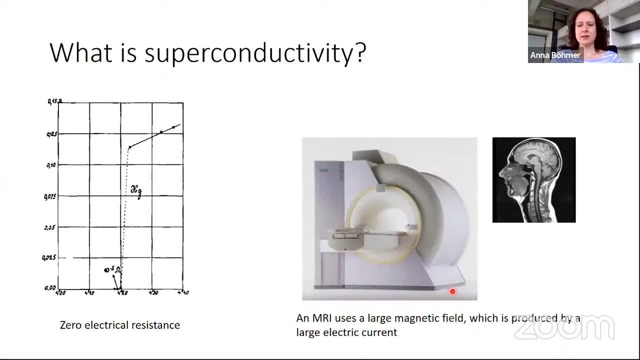 resonance imaging, medical imaging. what we need for that is a high magnetic field. to get a high magnetic field we need a large current. if we drive that through a superconductor, that's what we get. if we would drive that through a normal metal, we would not only get a large field, we would 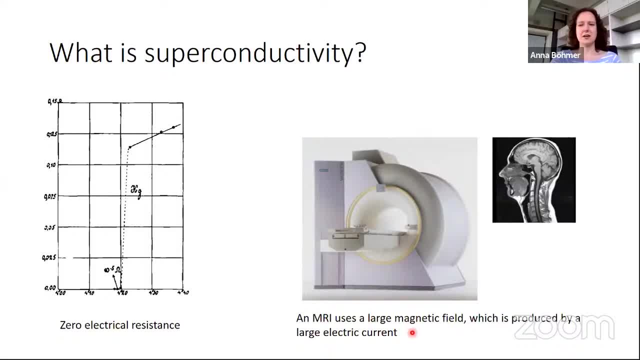 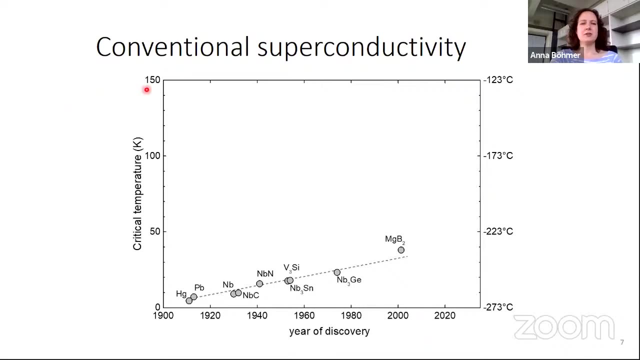 also get a lot of heat because of dissipation resistance, and then an mri would not be an mri, it would be a toaster. so it's the superconductivity that makes the difference. this is a famous plot of the history of superconductivity, a way to see it. what we 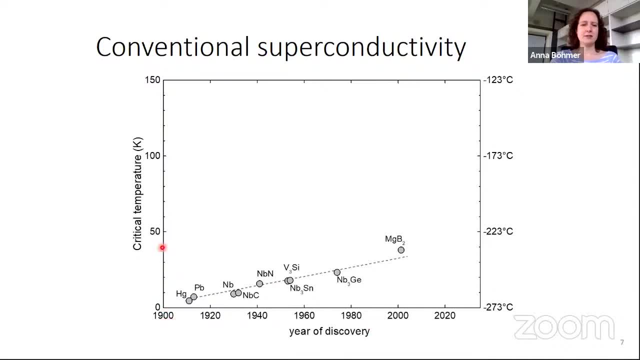 plot here is a function of the year of the discovery, the temperature below which a certain material is superconducting, and you see, over 100 years there have been- well, there have been- a lot more materials found, but this is the highest tc ones and highest critical temperature ones and there is an increase, but it's small. 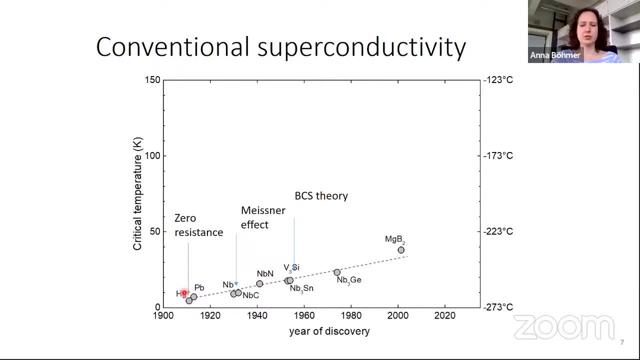 to this plot you can add milestones of research, the discovery of the zero resistance. there is an effect called meissner effect, about the behavior of a superconductor in a magnetic field. there is a theory that explains this effect. it's actually a triumph of condensed matter theory. 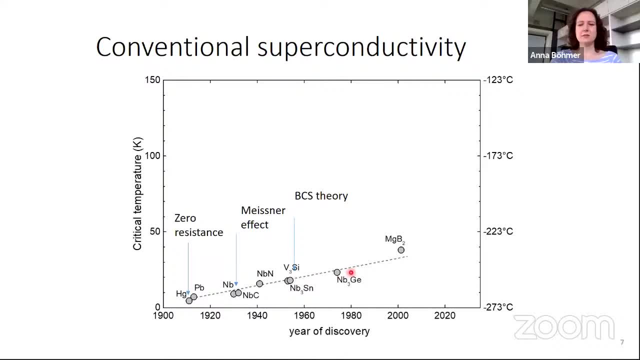 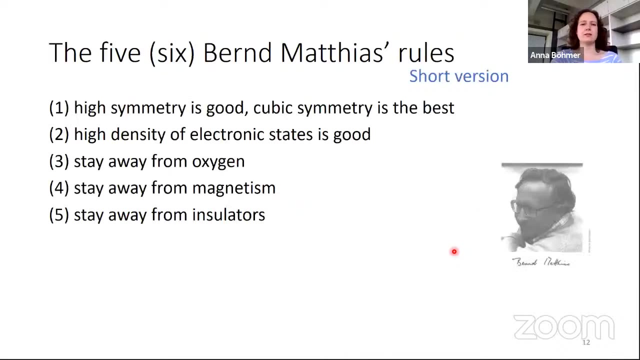 but you can see it did not help us getting higher tc materials. so this just continues. over this period and with all of these materials in mind, a couple of rules have been established for how to find a high temper, a good superconductor, and they are the famous burnt materials. so in a short version they say: try to look for super connectivity in. 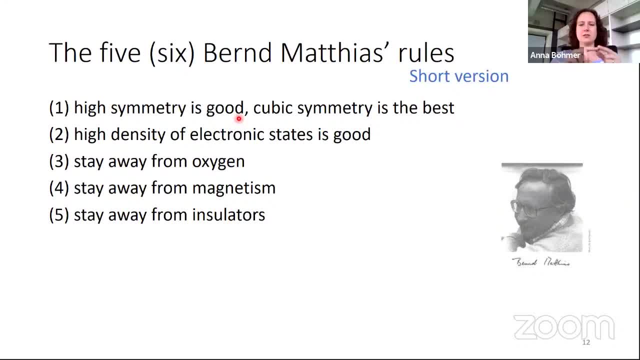 a high symmetry material, ideally a cubic material. it's the same along all directions: high electronic density of material. its very peculiar, in Victor De La Corretta's case, was the electric of seriousness as to where is the laminar mass of folk material, the auroral point жд attendance agent. 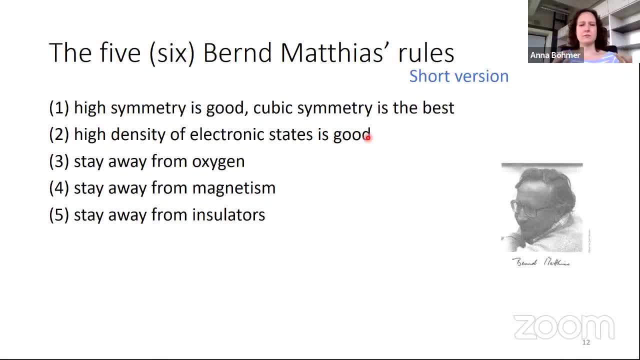 states also helps. So lots of electrons at the Fermi surface, Lots of states for electrons at the Fermi surface. Materials that contain oxygen are not a good idea. Materials that are magnetic are not a good idea. Insulators are not a good idea. And there's an apocryphal one. maybe Don't. 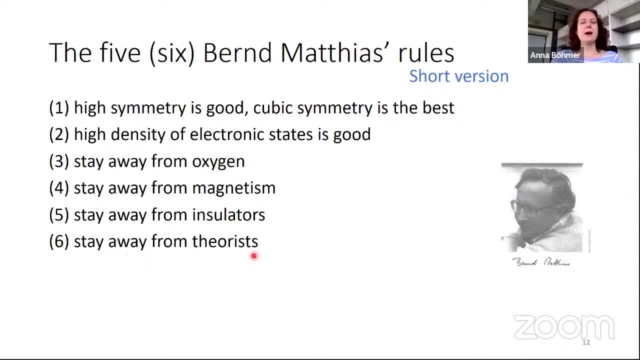 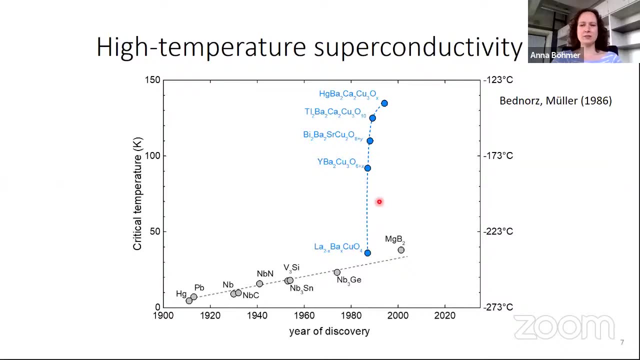 listen to the theorists, They cannot predict it. So that was established and that helped to find a lot of these materials. And then in 86 there was a discovery That was the cuprid high temperature superconductors, And you can see this enormous increase in critical temperatures. So now 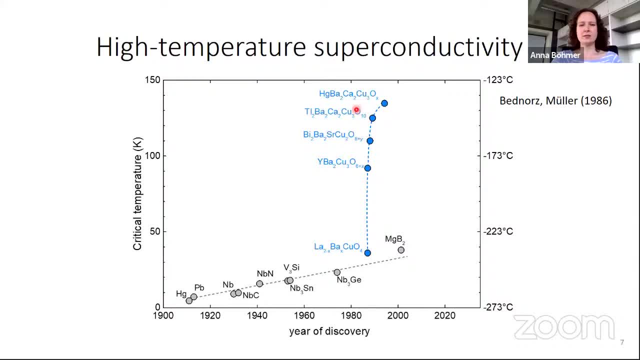 suddenly we have a superconductivity that's superconducting below 130 Kelvin or more. That's huge. That was a revolution. What happened here? Well, if you look to the materials we learned, we found a lot of these materials And then in 86, there was a discovery That was the. 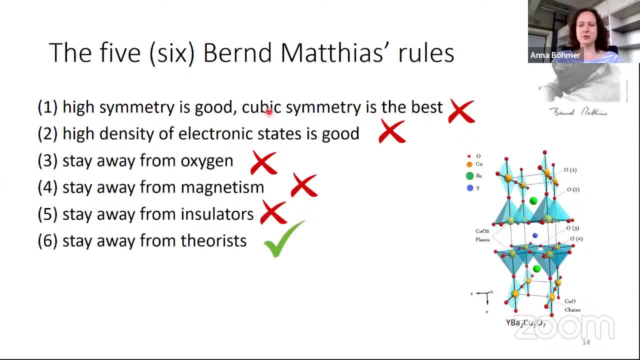 basically violated them. These are not cubic materials. They are very much two-dimensional, Basically the opposite of cubic. There is a very low electronic density of states. They are oxides. Here's an example: They are magnets, at least in their undocked state. But there's magnetism there. They are almost insulators. 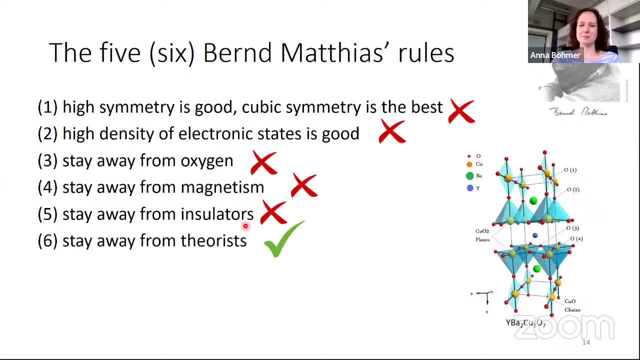 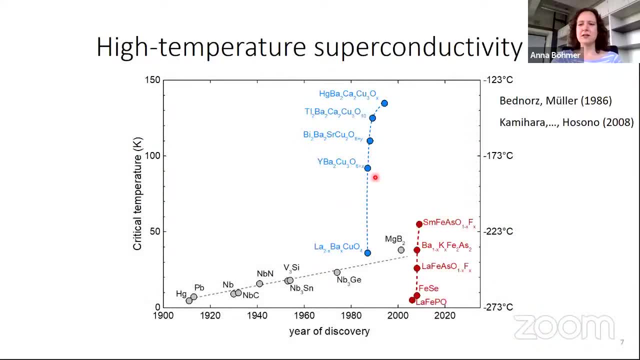 The only rule that's still valid is: well, the theorists could predict that, So that one still works. So, after the discovery of the cuprids, another class of high temperature superconductors is these iron-based superconductors. That's the one that I will talk about later in this talk. 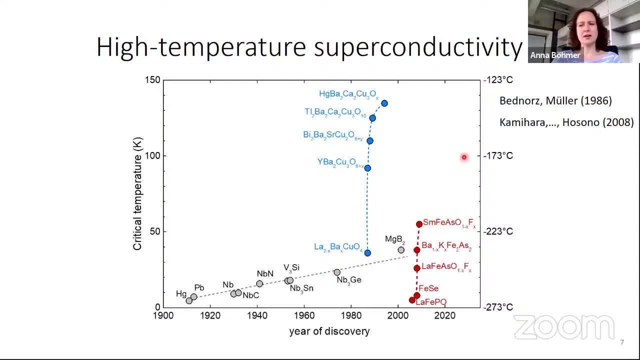 You can see, the critical temperature is not quite as high. But, as you will see, they are also very fascinating. One aspect that's fascinating is their phase diagrams. So this is a phase diagram, a temperature and a tuning parameter to the right. 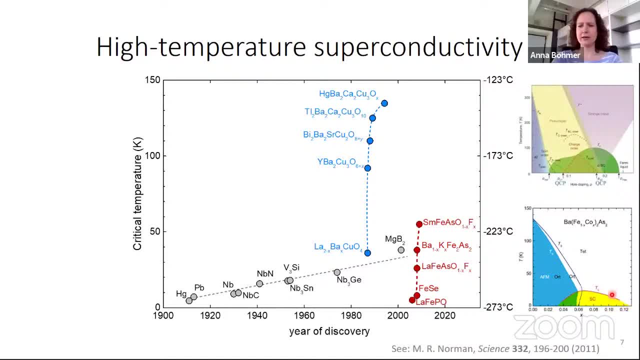 What you see is a superconducting range. That's the green part here, It's the green yellow part here. What they have in common. there is something else around here or here. So if we look there and if we look at, if we think about the introduction, that looks similar. 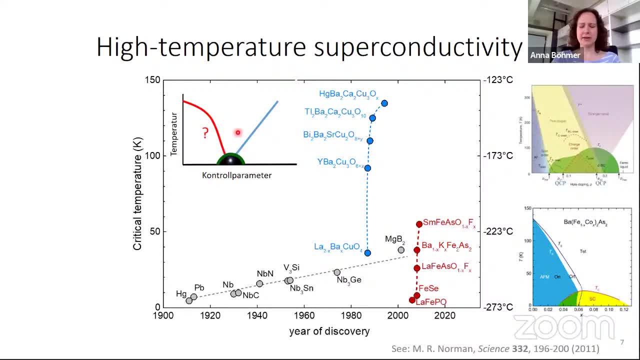 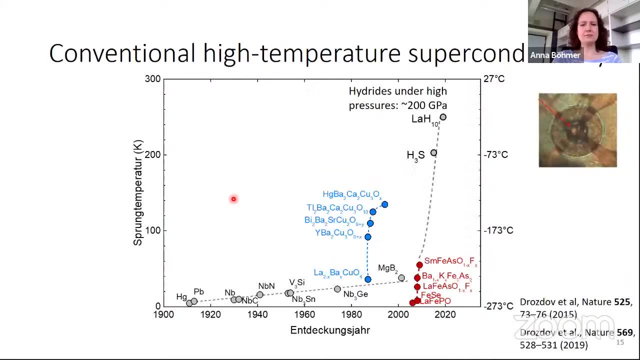 So a new paradigm is: well, we want to look for magnetic phases or other phases that are suppressed, and around the point where they're suppressed, maybe that's where we find our interesting superconductor. That is a fruitful way, But it's not the only way. So now I have to change my scale on my history plot. 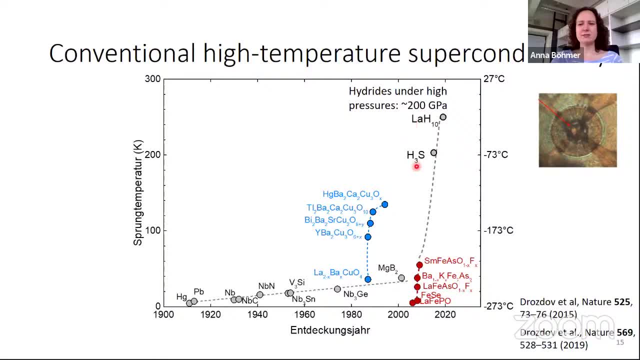 That was only a few years back. Superconductivity was found at well, almost like almost room temperature. It's not quite room temperature, but this is a outside temperature in winter in Siberia, for example. The drawback is this is superconducting at only a high temperature. 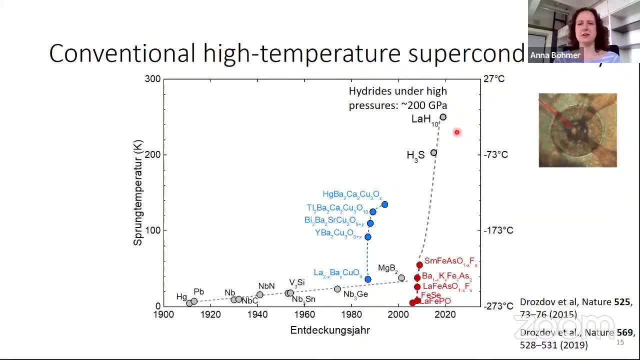 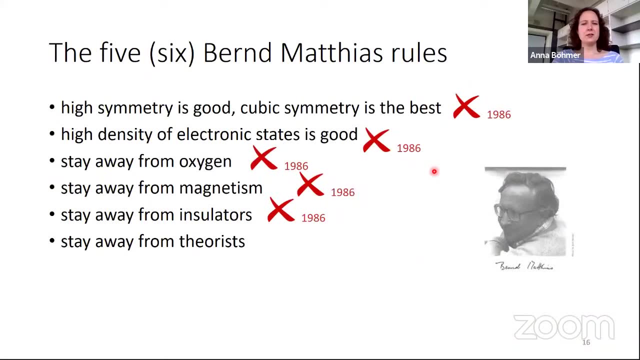 200 gigapascal of pressure. so that's very far from atmosphere. So applications are still far. but fundamentally we have found a really high temperature superconductor here and these high-dress materials. What we go back to our rules now. we know these rules well. they don't. 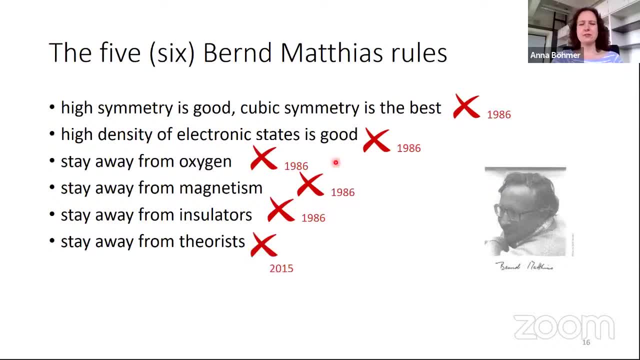 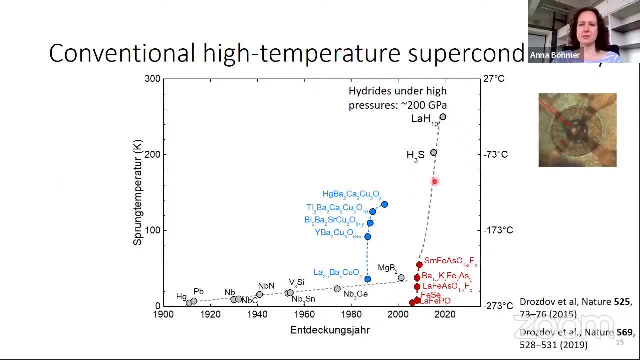 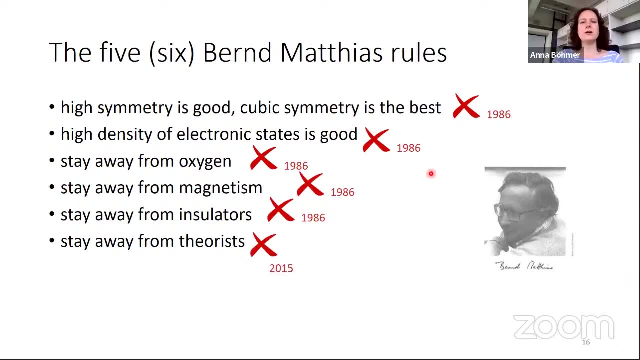 didn't work for the 1986 discovery. For the 2015 discovery, even that one is violated. The series did predict it and it was found experimentally only later. So the series said: look at this. at high pressure and high superconductive temperature, superconductivity was found. So with this, let me 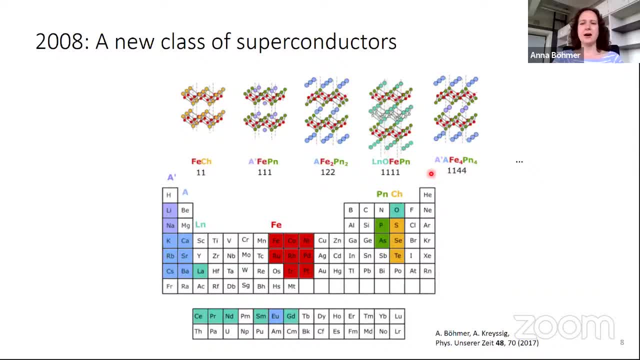 come to the class of superconductors. I have been working on The iron-based superconductors And one thing that's really fascinating about them is we have a lot of them. We have different materials, There's some abbreviations here. They all come in different chemical structures. What they have in common is iron and red here. 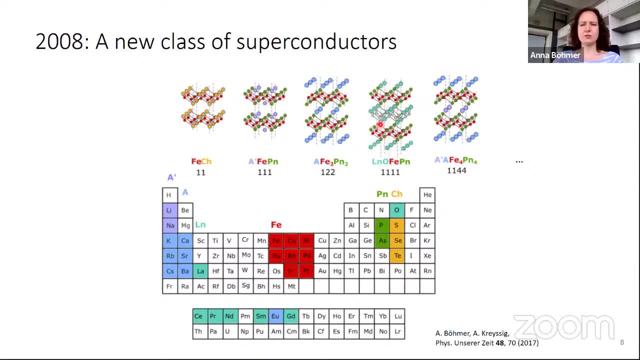 and then typically arsenic, sometimes phosphorus, around them in layers, But we can use many other elements as well. So there's a good part of the periodic table that can be taken, built according to these structures, and every time we find a superconductor. That's quite amazing. So there's 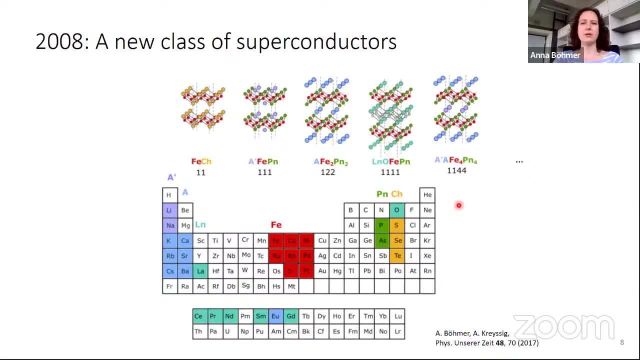 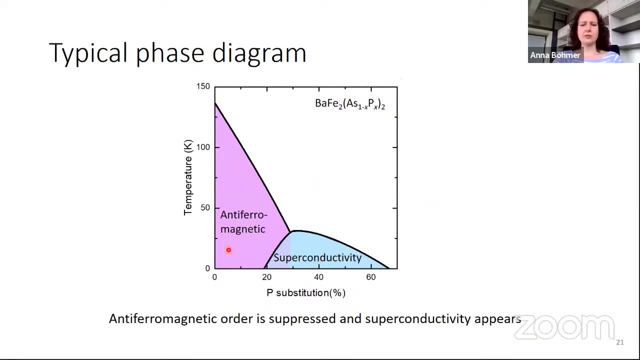 a lot of tuning parameters, even a lot of chemical tuning parameters we can play with, And let's look at a typical phase diagram here. So again I have temperature. Now I have chemical composition here as my tuning parameter. The material specifically is barium, iron, two arsenic. 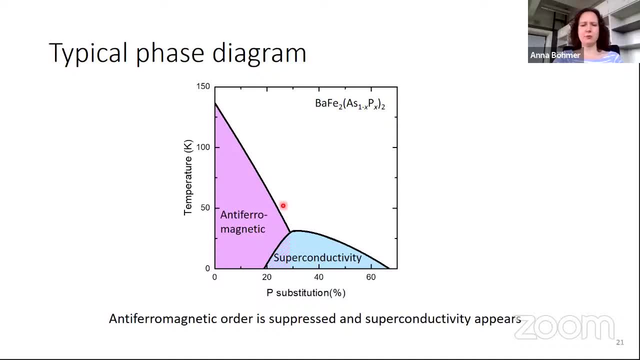 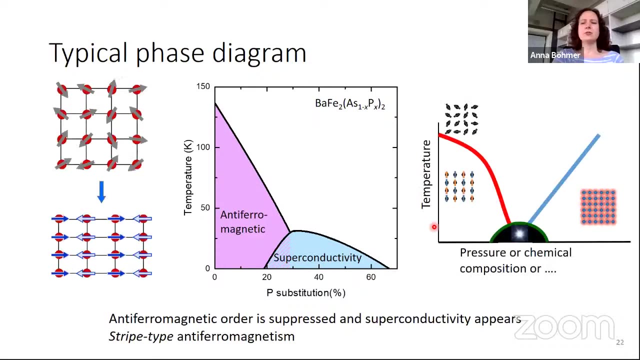 two and then a little bit of phosphorus in there. What we find is an anti-ferromagnetic phase and a superconducting dome, Very similar to that suppression of magnetism and a new phase emerging As in the introduction. So the question here is- and the question that we are very much interested- 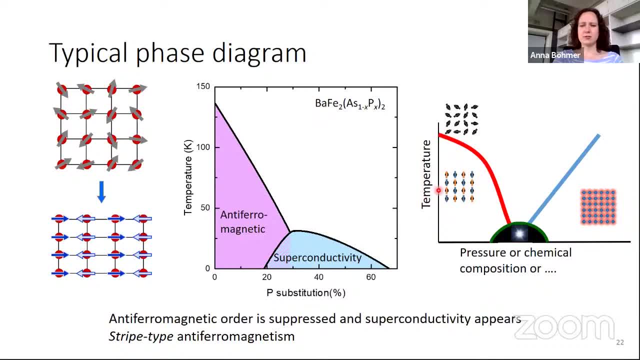 in. What is this phase that is suppressed to get the superconductivity. And here we have a magnetic phase. We have an anti-ferromagnetic phase, which is a little bit special. What we find is the magnetic moments, which are disordered at high temperature. They point in any direction. 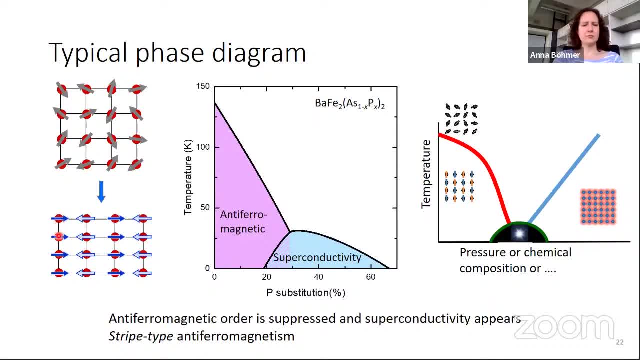 They order in this way that they are parallel along this one stripe and then anti-parallel to the next ones. So we have a stripe type anti-ferromagnet, So basically a ferromagnetic direction and an alternating direction. That has interesting consequences. 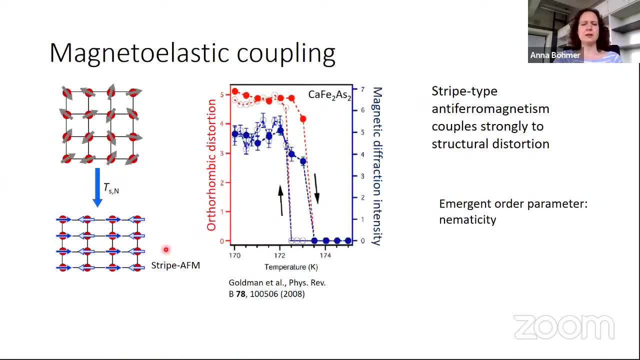 which I will explain in a bit. One of these consequences, as a preview, is magneto-elastic coupling. So now we couple the magnetism to an elastic property. So if we go from this state to this one, We go from something that's well a square here, The material itself. 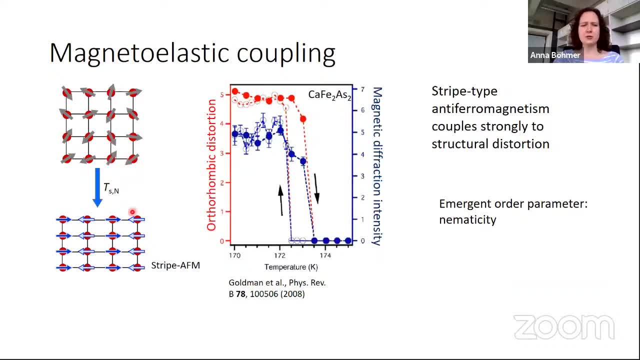 it's called tetragonal, But the iron net is just square To something that is no longer square Because this direction is just different from this one. So, just by symmetry, this cannot be a square, A perfect square. at least, If we measure this, we find it's not a perfect square. So here is function. 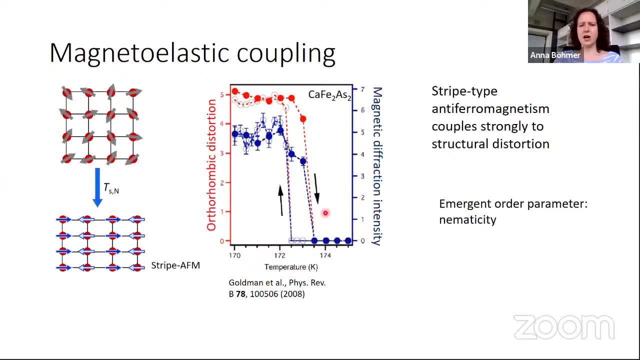 of temperature. We look at the magnetic Well, basically how much the magnetic order there is in blue And how much this deviates from being square in red, And that just goes hand in hand. So we find a strong coupling between this sort of anti-ferromagnetism. 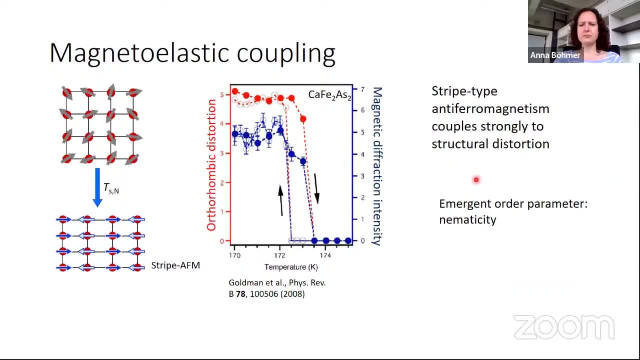 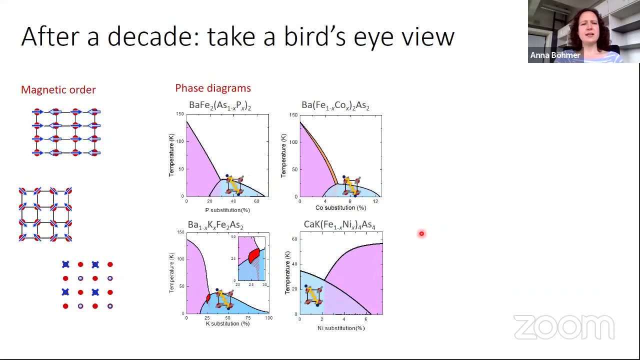 to a structural distortion, Distortion from square. This goes with what's called an emergent Euler parameter, And that's going to be at the end of my talk. I hope I can explain this interesting concept of solid state physics. But after a decade of research now, this was discovered. 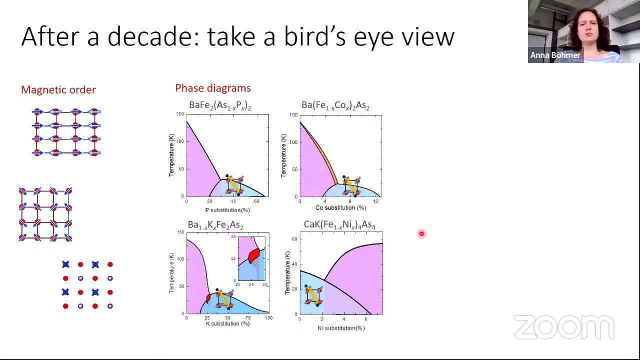 in 2008.. I think it's time to take a bird's eye view and to see what's there. What can we understand by looking at many materials, many properties, And what I will find, and what I will show you, is different sorts of magnetic order, A couple of different phase diagrams and different 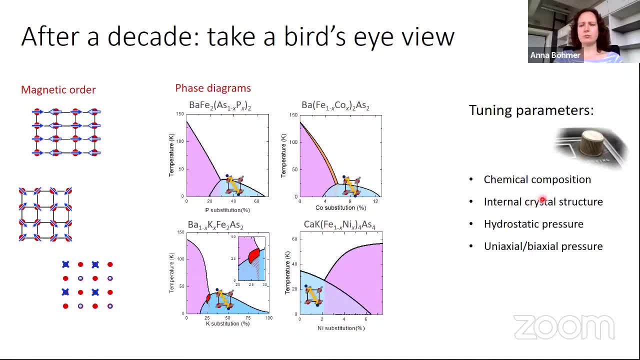 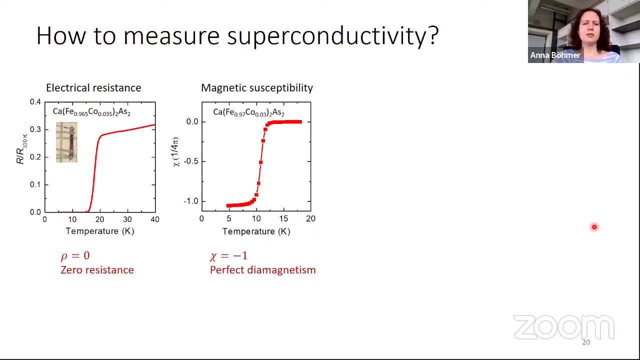 depth, articularities And a couple of tuning parameters. We had chemical composition, We already talked about hydrostatic pressure, But there are a few more. But when we do our experimental research- And this is really data that I've taken- One question is: how do we see super connectivity? How do we measure it? 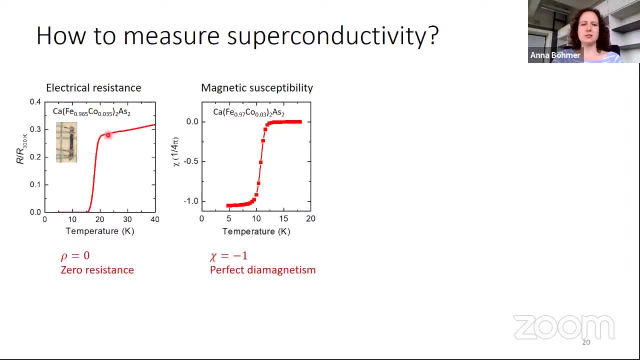 And we do nothing else than come running on us And we measure electrical resistance. We put four contacts on a sample, We measure the voltage we applied to the sample. And well, voltage on a sample, The current, And we find zero electrical resistance below a certain temperature. 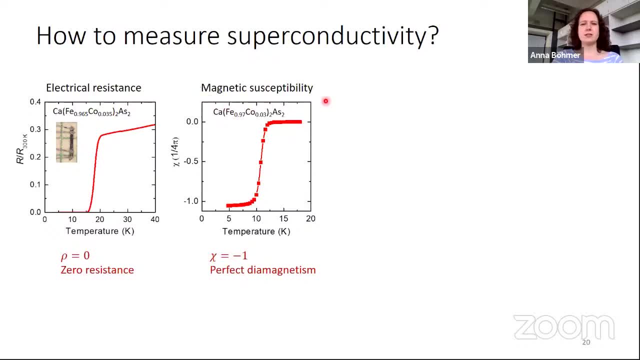 We also measure magnetic susceptibility. That's this Meissner effect that I've briefly mentioned. It's the property of a superconductor to be a perfect diamagnet. But well, there's machines to measure it. You need to understand better what they do. But what you find in the end is a diamagnet Here, Below a certain temperature. 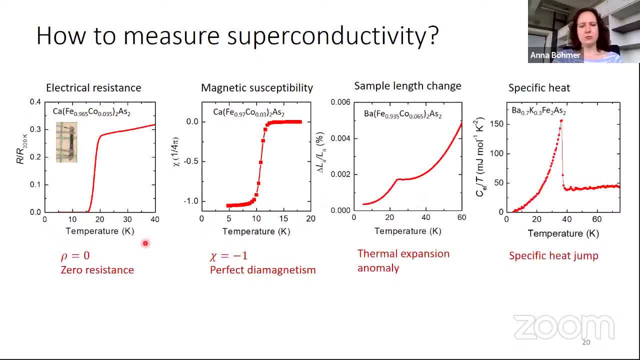 And there's other things to measure on a superconductor. These two, Well, that's just the definition of super connectivity. These other things, they tell us something more. One of them is the sample. The sample lengths change on going through a superconducting transition. So here what I plot. 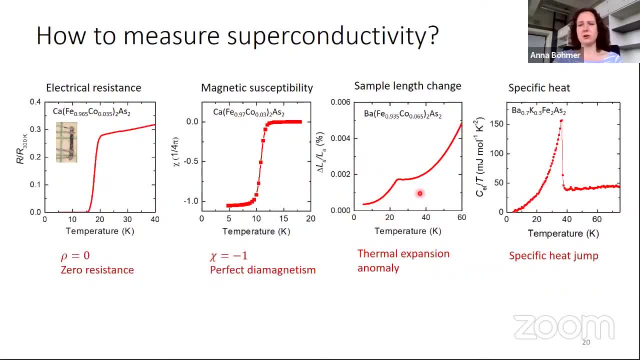 is, as function of temperature, the length change of my sample. So, like a piece of copper, It shrinks when you cool it and expands when you heat it up. A sample, Any sample, will change length when you change temperature, But when you go through a superconducting transition, And that one is here- 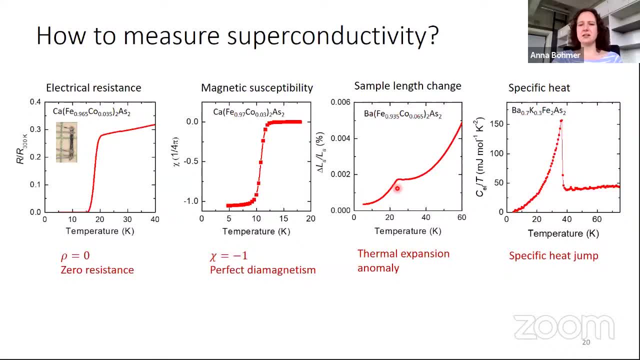 This length, change will change. So really you can see the fact that the sample, The electrons in the crystal go superconducting The electrical resistance in the sample length as function of temperature. That's what we see here. That's, if you think of this, This is a quite amazing. 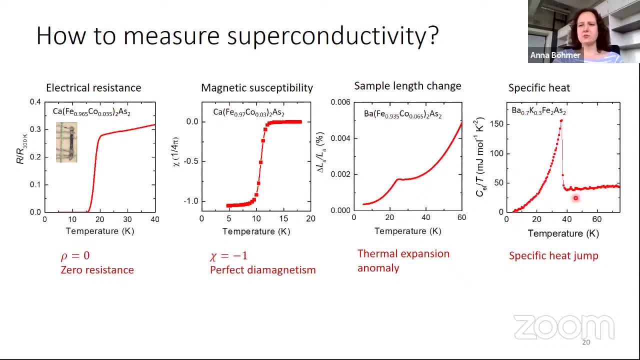 Another property is the specific heat. So how much, How many kelvin, How many degrees the sample heats up if you put a certain amount of energy into it, And there there is a huge change. also at the superconducting transition This has to do with electronic order and the entropy that's. 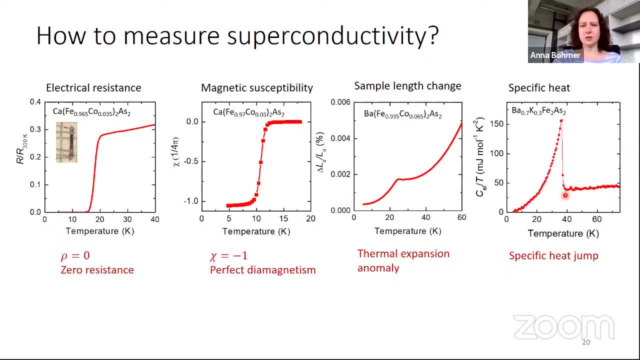 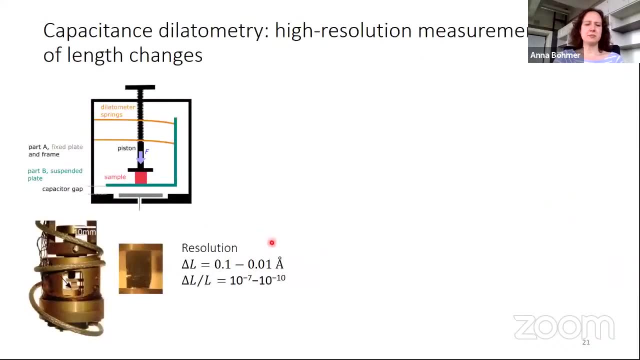 lost there. It's also an important feature of a superconductor And we can learn something from how large this change is. And let's see what we can learn from this In a bit. First, I had my measurement setup, Or one of my measurement setups, The one that I like. 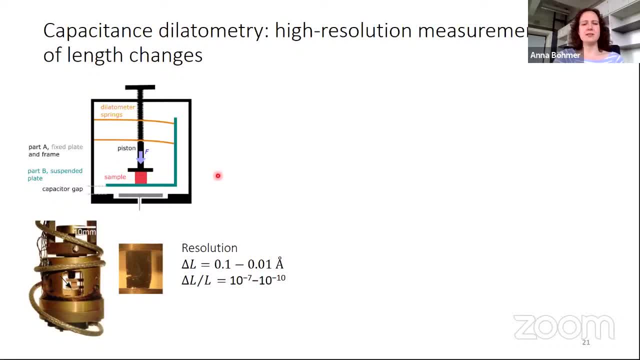 most. actually It's a capacitive stillatometer. This is something to measure length changes with high resolution. The principle is easy. We have a plate-type capacitor, So the capacitance- you learn that in elementary physics- depends on the distance between two capacitor plates. The magic and the trick is to couple the distance between. 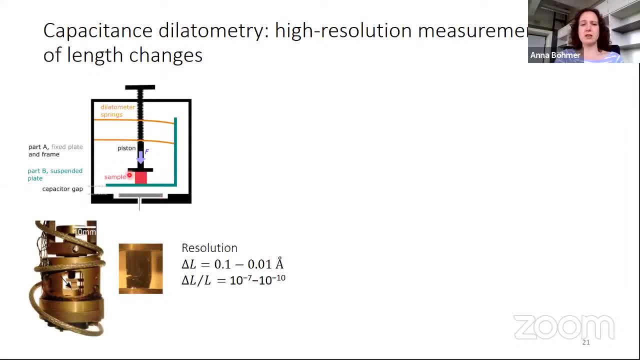 these two capacitor plates- They are found here- To the length of a sample, And if you do that, all you need to do is read out the capacitance to get the length change of the sample. We can do that with very high resolution. We can see length changes of fractions of angstrom. 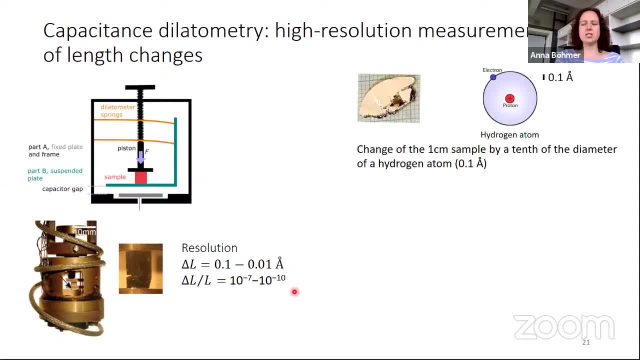 Just to remember, Just to find pictures for how much that is. It means that if our one centimeter sized sample changes by a tenth of the diameter of a hydrogen atom, That's point one. angstrom, That's a change that can be seen, Or try to find macroscopic. 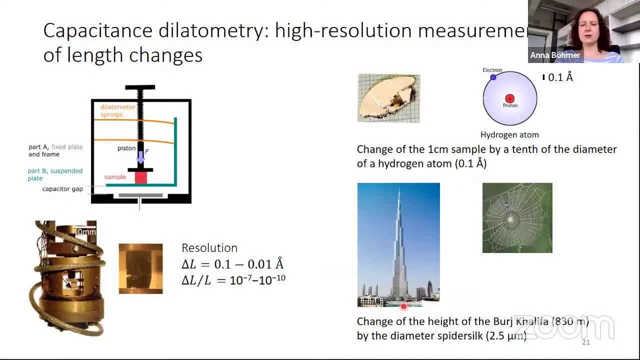 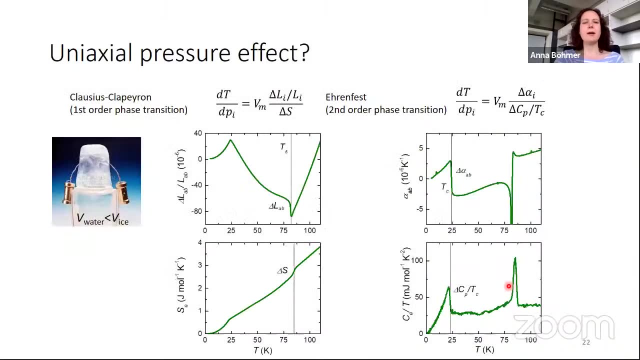 examples. It's as if the height of this highest building in the world, in Abu Dhabi, changes by the diameter of spider silk. That's a length change that can be seen And that's something we can learn from superconducting properties. And what is that? One thing we can learn is: 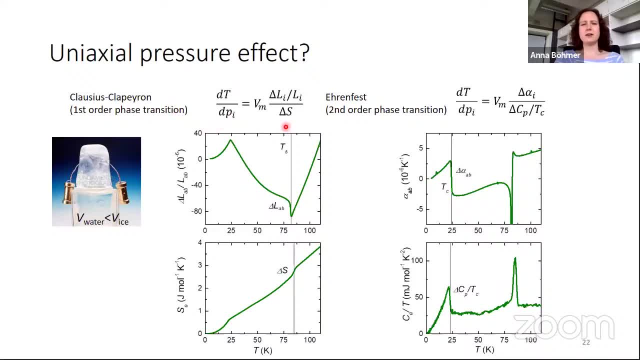 uniaxial pressure effects. So this is a basic thermodynamics. You might have seen that before. What it tells us? the relations are quite famous. One is Clausius Clapeyron. What you say is that the pressure derivative of a certain temperature is given by the length change of a sample. at that, 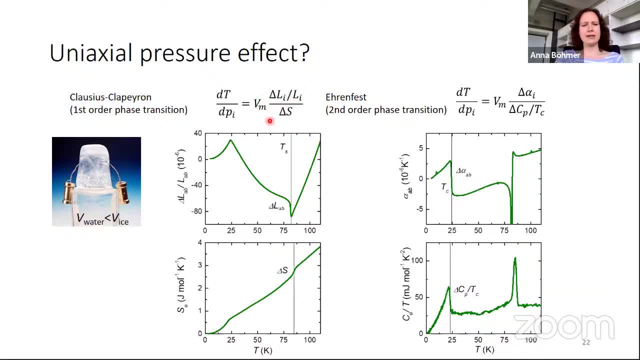 temperature Or the volume change, Divided by the entropy change, You can see that with ice It's quite intuitive. Well, ice has a larger volume than water. So if you compress ice, you'll melt it. It wants to be water, It does not want to be ice anymore. 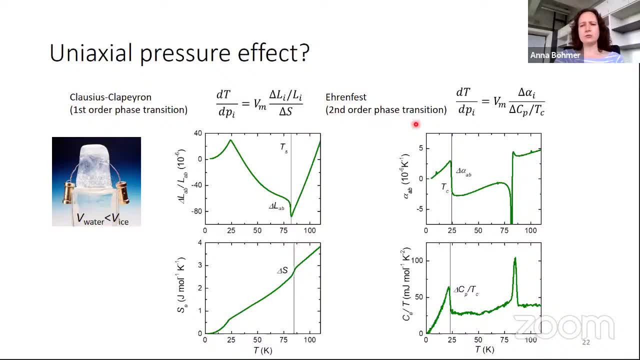 That's what this relation means. You can do it too for so-called second order phase transitions. The length changes where there is rather kinks in the length or jumps in the derivative of the length. That's this alpha, And then it's called Ehrenfest relation. 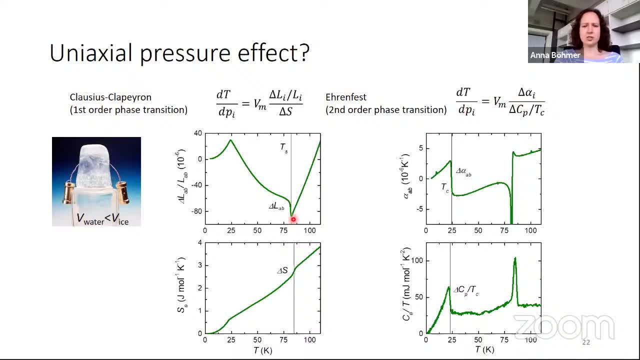 Here are some examples. At this transition, the length or the volume increases suddenly, The entropy decreases suddenly. I take the ratio of the size of these anomalies and I get the pressure derivative Here. that's a superconducting transition. actually, This expansivity increases. 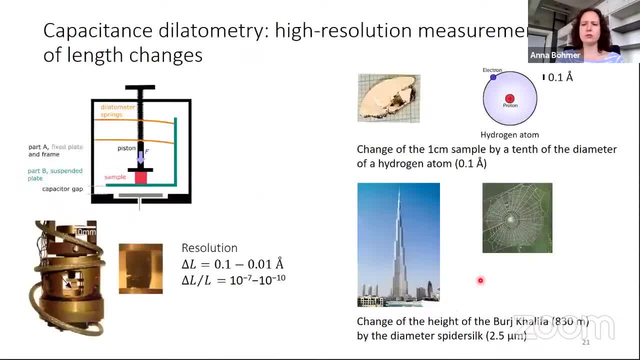 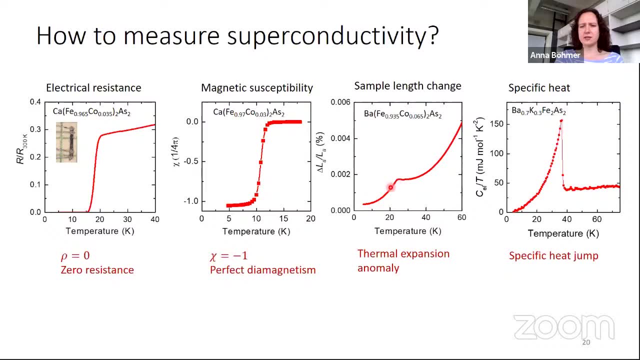 and the specific heat increases. Let me just go back to show you where this comes from. So this was the length. at a superconducting phase transition. It doesn't jump, It has a kink. Temperature derivative of this will be a sudden change. This is very steep, This is very flat And that's. 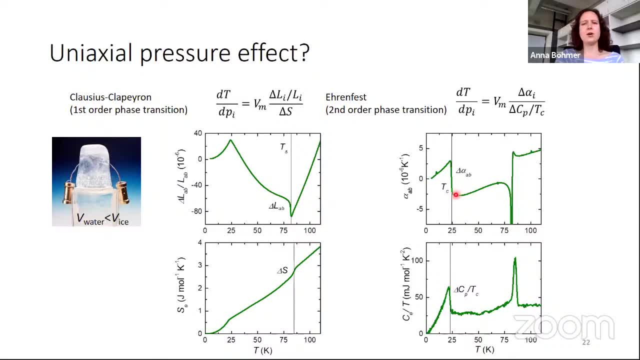 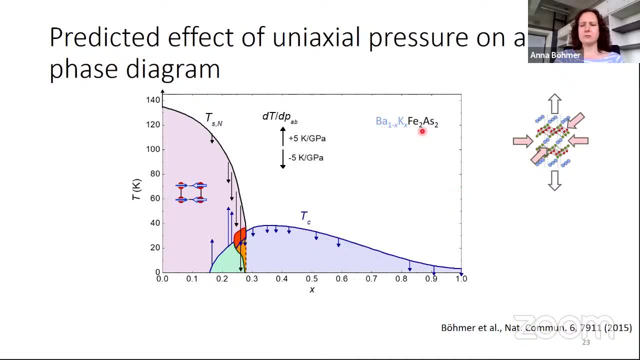 exactly what goes in here. If we do that, what can we learn? This is what we learned for one of these iron based materials. What we I show here in terms of arrows is over the phase diagram. This is a magnetic phase. This is a superconducting phase. 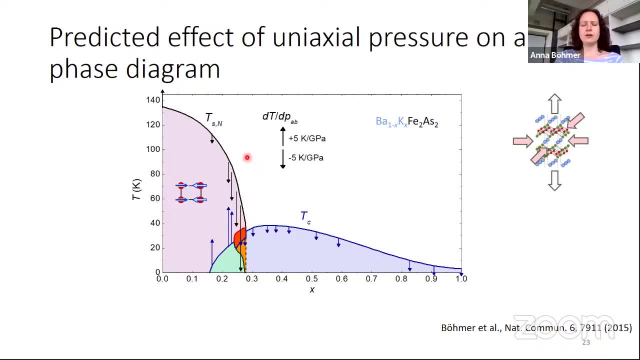 There are a couple of more phases here. what we learn is, at a uniaxial pressure in the plane symbolized here, this transition temperature will go down by this much, and this one will go down by this much, this one will go up. so summarizing this way: on the other hand, we did similar measurements, but now for c-axis. 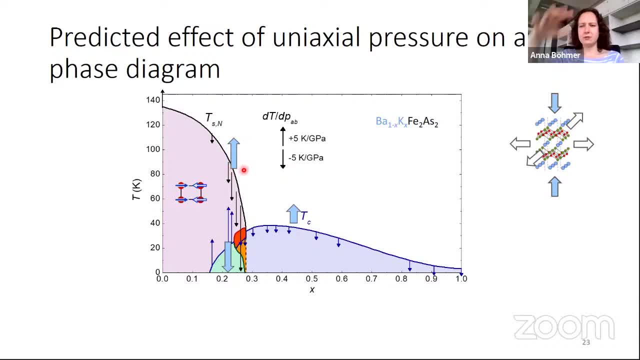 direction. what we learned there is, for if you compress the material along this other axis, this temperature will go up, this will go down, this will go up. so there's a sign change here, everything's opposite. so what we can conclude is that the best tuning parameter is neither. 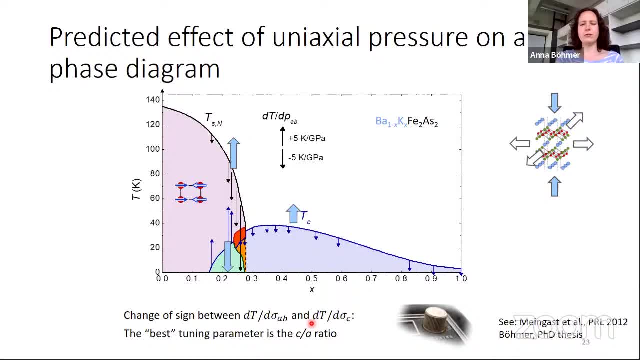 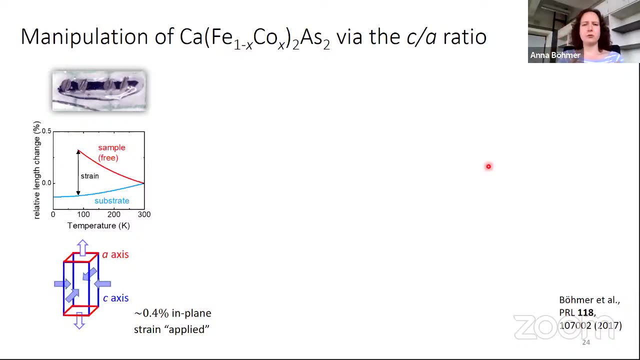 this pressure, not that pressure, but it's the difference of the two, or the ratio of c over a, the ratio of this length to this length. that's the best tuning parameter and we have used it to change the c over a ratio externally, like voluntarily. you, you need to. 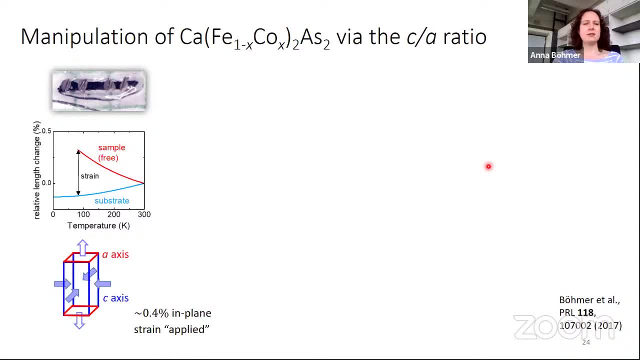 play a few tricks. that's not so easy. one trick that we did is we have a sample and we put it on a substrate. substrate is glass. here it's really just a piece of a microscope slide to cover glass. um, and we know this thermal expansion of sample and glass. 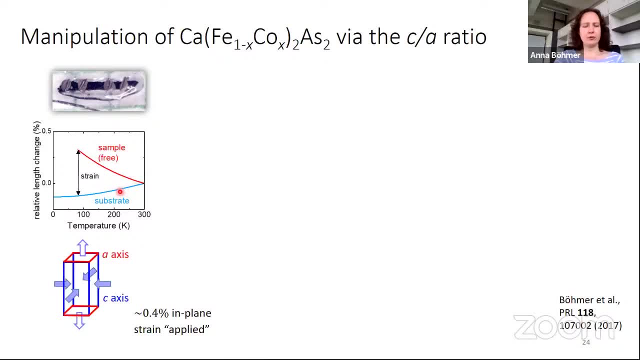 it was measured. so the glass that's. that's a regular curved thermal expansion. you pull it down from room temperature, it shrinks by a few, a little bit fraction percent. our sample, it turns out, actually wants to expand on cooling. it's negative thermal expansion that happens. 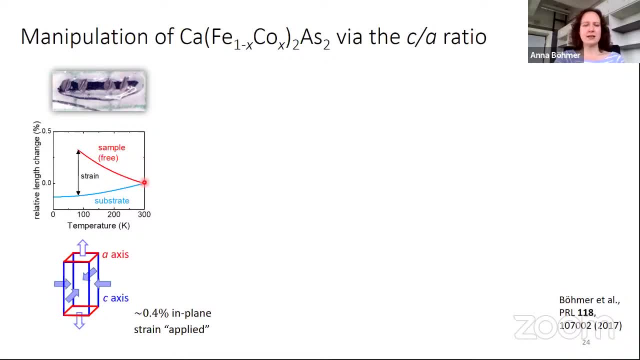 but this also means that if we have a sample on glass, it wants to expand but it can't because we fixed it to it. so what we are really doing is we compress it in the plane, the c-axis, the other dimension. up here it's free. so if we compress something that doesn't want to do, 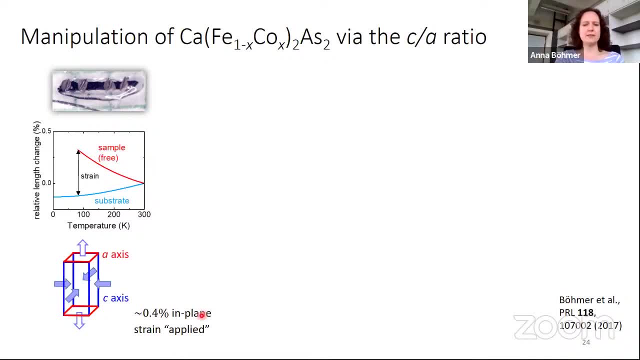 it, it will expand in the other direction. so we are really changing the c over a ratio here. and what happened? what we saw is: okay, this is basically a sampling, but measured using x-rated fraction. what we see is a transition as function of temperature from a single peak to a double peak or 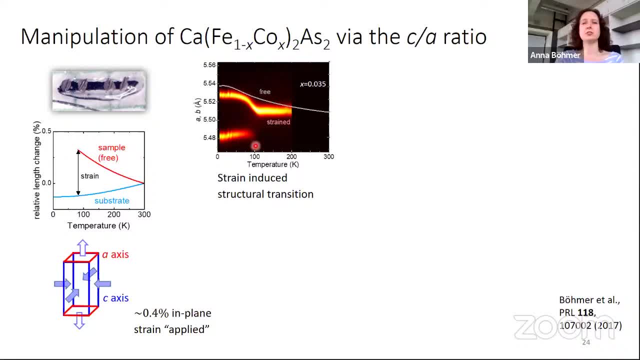 from a single lattice coefficient to a double lattice constant. what this means is there was a structural phase transition. actually, here this was a square and now it's a rectangular lattice. that's what we see. you also use the different technique. that's a most power spectroscopy. don't really need to understand it. 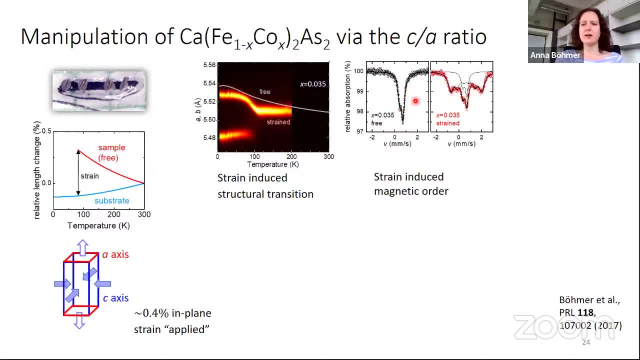 it means. well, we see two very different spectra at for a free sample compared to the sample on the substrate. here the sample on the substrate is a complicated spectrum and it means it's magnetic. there is magnetic order these moments. they have ordered and we also measured this magnetic. 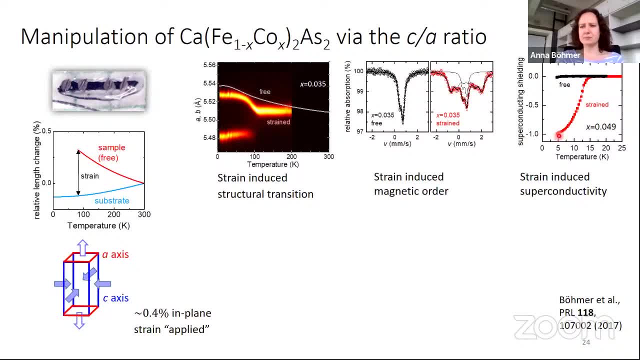 susceptibility and we find a diamagnet in the sample, on the substrate, in the strain sample. so it's a superconductor now when it wasn't before. so we've tuned the material via the c over a ratio and if we put all of it together, what we've done is we've manipulated the phase diagram. we went for something like this turns out: 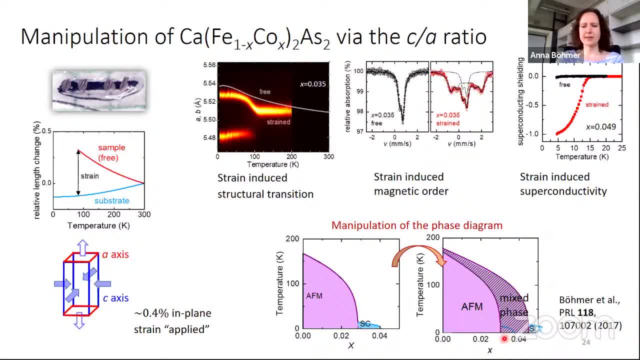 to something like this, using the C over A ratio. I have indicated here a mixed phase, something special that happens, and to me it was an example that you really need to think carefully and you should be open to surprises of what happens. And this is well thinking about it. 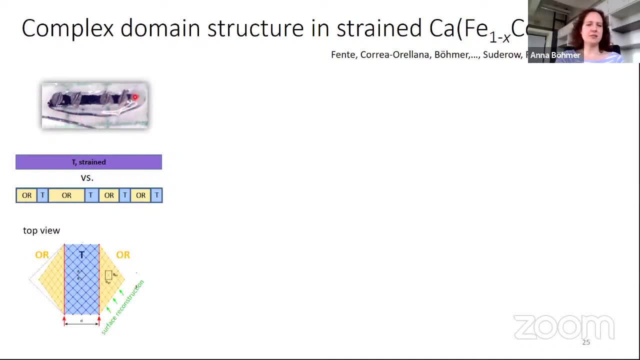 carefully. If we thought about this carefully, we have a sample on a substrate that is T stands for tetragonal, like before my transition, but it's strained, it doesn't have the length it wants And it turns out, instead of staying that way, what it wants to do is it only goes partially through that phase transition We have. 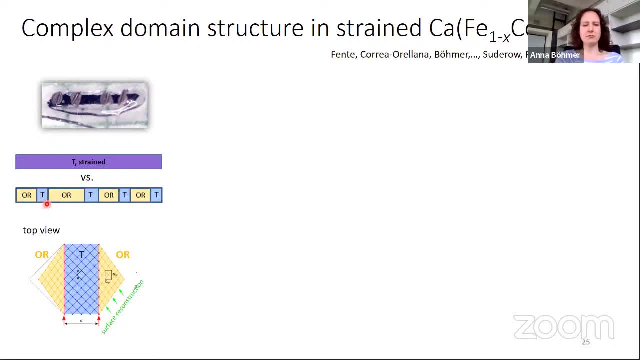 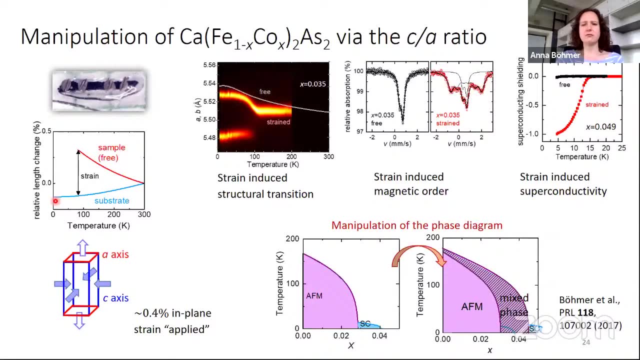 then some regions that are not strained and above well, without going through phase transition, and other regions that have gone through that phase transition. By that phase transition I really mean in that structural one here. So we have part of our sample that's here and a part 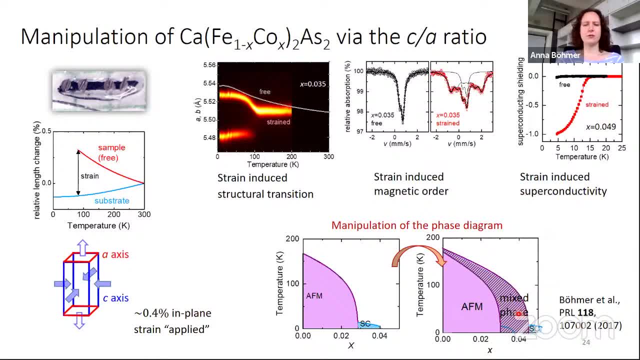 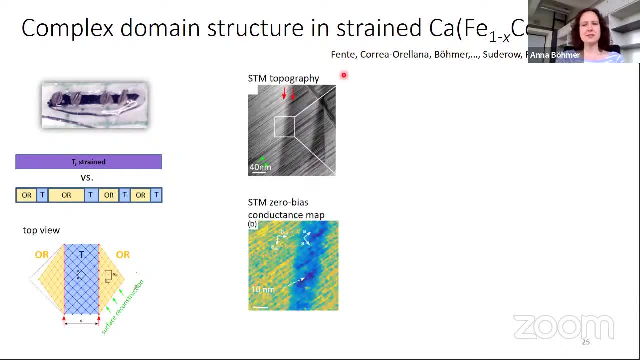 of our sample that's here all over the phase type, well, all over the mixed phase, And that was or. Hermann saw it together with Anton Fenter in STM. So he looked at this and he sees different regions and these will be these different regions And if you want to know if it's a super 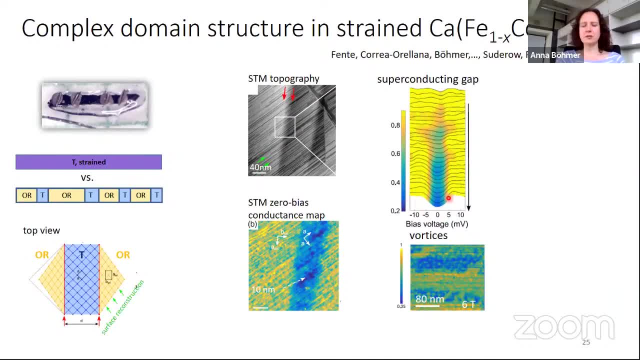 conductor. you can do a what's called spectroscopy And from the spectrum you can see this region is really a superconductor and the other one is not. You can also look at: is it a square lattice or is it a rectangular lattice? Did it go through? 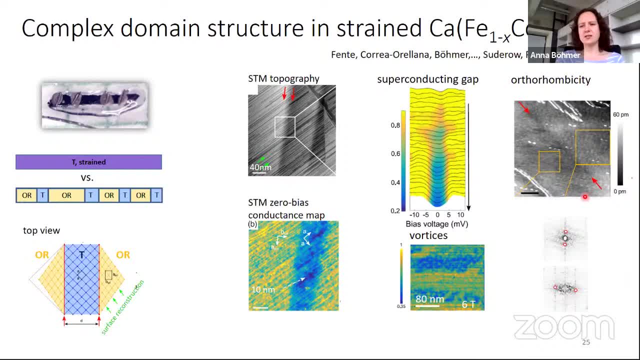 the structural phase transition And then some parts. actually, yes, they did So what we find here is a really nanometer scale, very small, interesting domain structure of the same material beyond different phases being different states. One of it is this osirambic, this distorted stripe type, and the 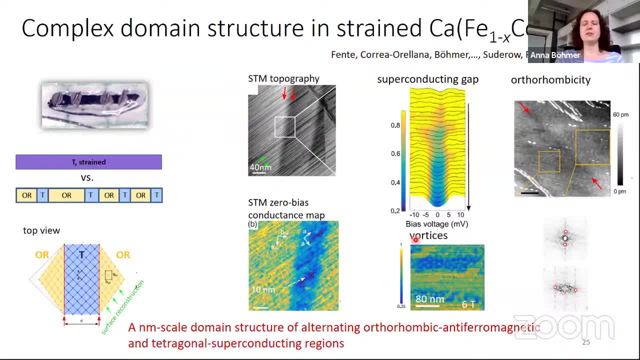 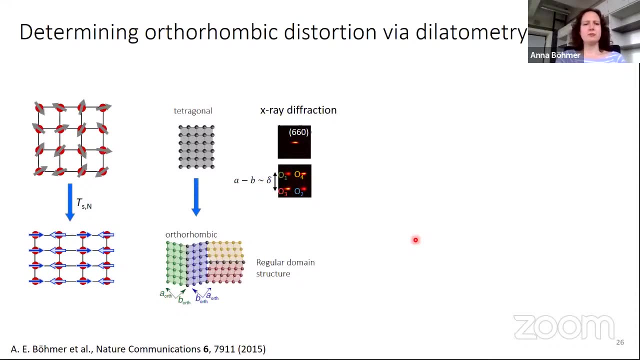 ferromagnetic one and one is superconducting. That's quite cool. Maybe we can think of some, some interesting consequences there Then. okay, I'm going slow here, but I'll skip a few things. There's just some interesting things to talk about. One thing that we did is we measured the osirambic. 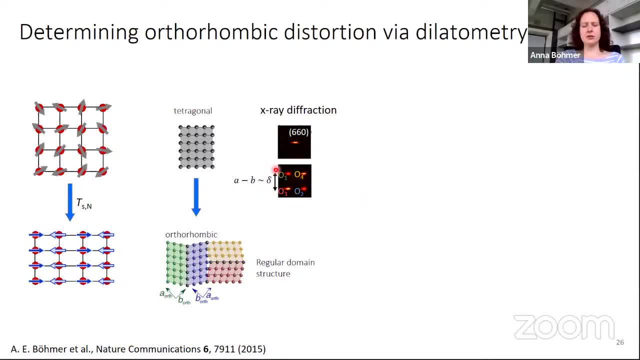 distortion using x-ray refraction. on one hand- that's what i already had- you see a set of peaks and the way they differ. that's how much your lattice differs from square, how much we go rectangular, how much we go in a magnetic state. you can also do that with length changes, if you. 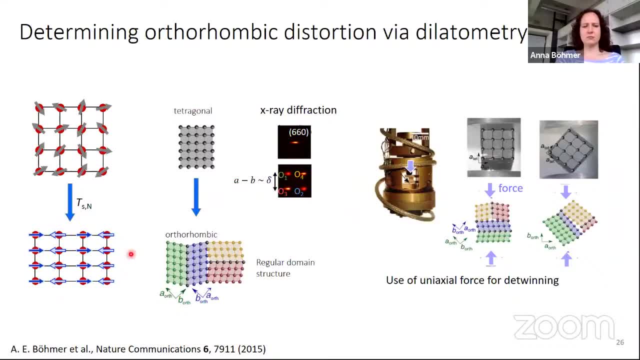 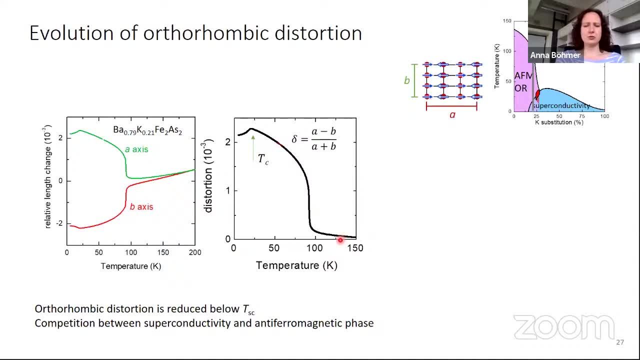 make sure you only measure this direction and not this. that's a short way. we did that. let's just say we did that. what we find is the orthorhombic distortion. the deviation from square is function of temperature in a bit of the phase diagram here. when we cool down, we go through the transition. we 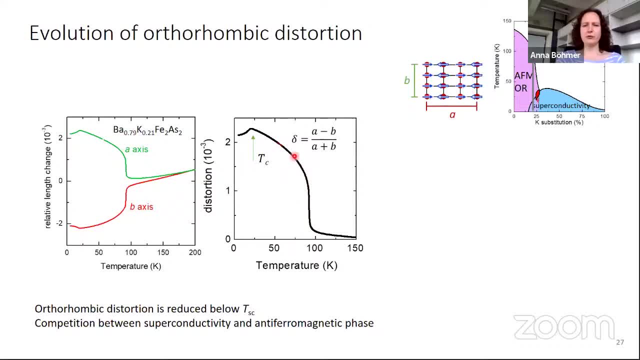 see the orthorhombic distortion come up. we cool down further and then we hit superconductivity and we see the orthorhombic distortion decrease. so here is another effect of superconductivity on the structure. so really, the fact that the electrons, they become superconducting, loose. 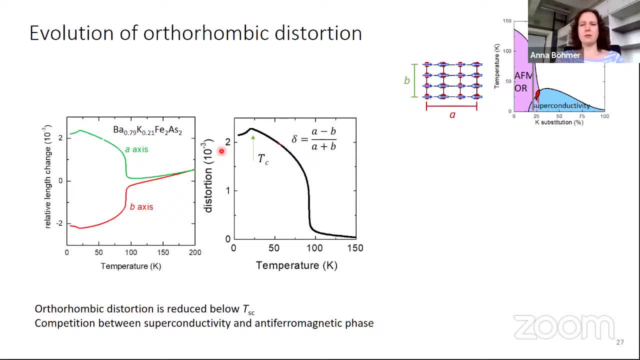 resistance means, or has a consequence, that my, my right angle changed shape. that was seen as well, and what it was seen by other people as well. um, and what it means is, or what we, we conclude from this is that the superconductivity and this anti-ferromagnetic described phase- they compete superconductivity. 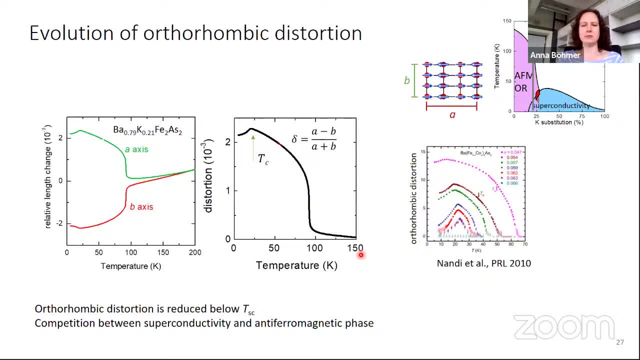 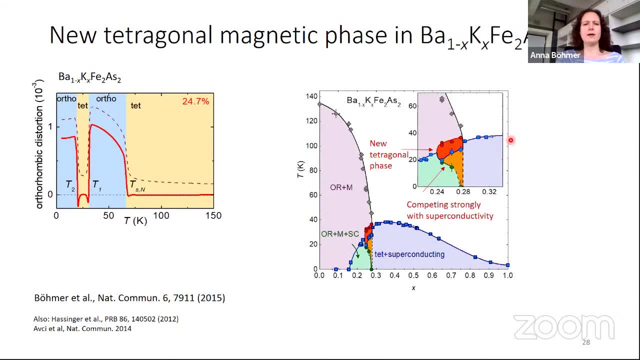 doesn't like the distortion and the distortion doesn't really like superconductivity. so we learned something about the relation between these two things. um, a surprising discovery made is we learned something about a new phase, that's this little red region here. when we did these measurements, what we find is an orthorhombic distortional. 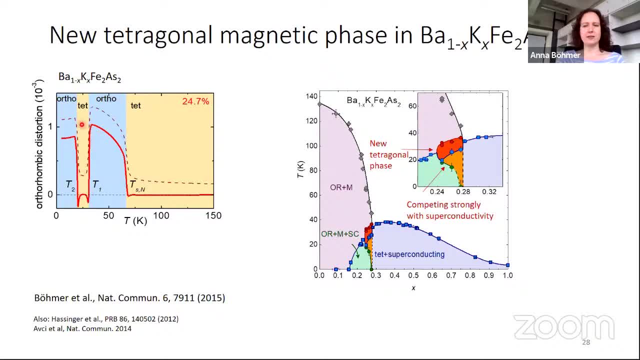 cooling comes up and then disappears and it comes back. and that was a discovery- or it was our discovery- of a new little face pocket in our phase diagram here, which was also seen by other researchers. um, but to us, seeing this curve, it was a real surprise and told about the power of this. 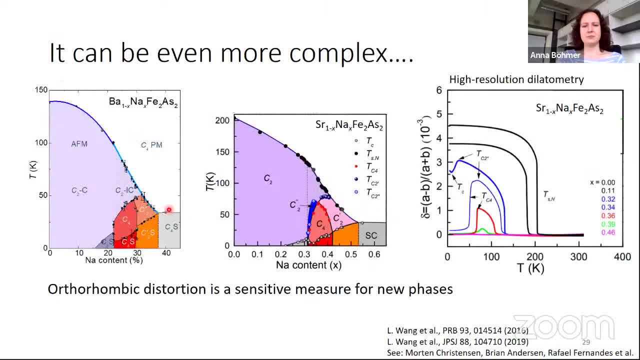 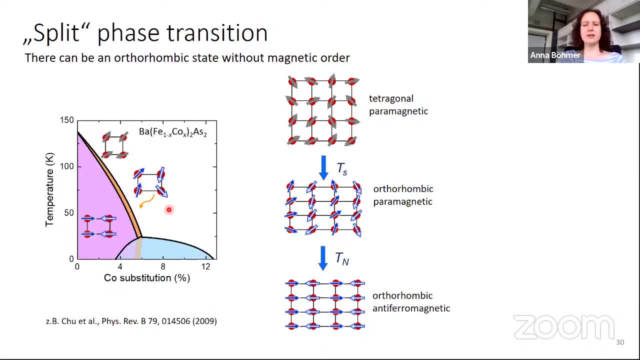 technique. um, there is even more phases discovered with this technique, which i will skip here just to, in order to come back to an interesting, one of the most interesting effects of this magnetism. here we have discussed so far the transition from this uh square, like the diagonal magnetically disorder, paramagnetic state to the stripe and a ferro state. 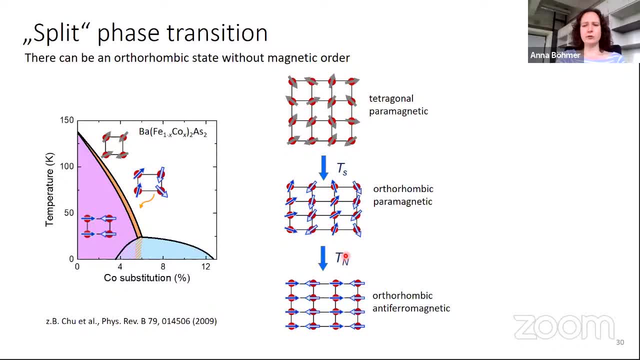 but it turns out- and this really was an experimental discovery at first- there can be an intermediate state, there can be a state that's no longer square, but the magnetic moments, they are still disordered. so if you think about it, it's strange, because we said this is no longer square. 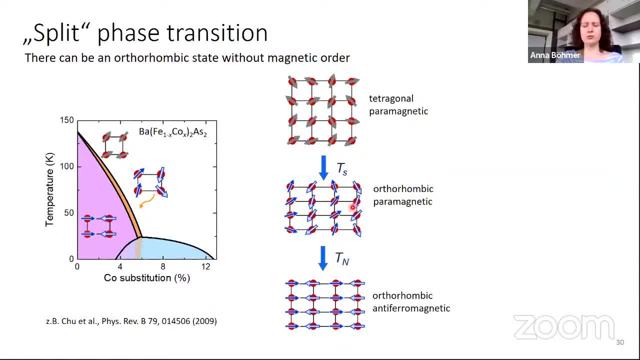 because of the magnetic order and our total magnetic moment is no longer square and we are- turns out- you can see this being no longer square- in a disordered state. What does it mean? Well, we worked on it and we found out. but first we need a name for that state, And it was named. 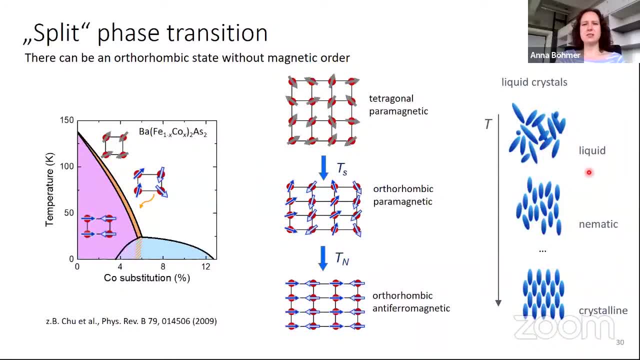 nematic in analogy to liquid crystal phases. Maybe some of you know liquid crystal phases just elongated molecules that can be totally disordered. They can be crystalline ordered but they can have an intermediate phase where there's sort of a directional order but not a 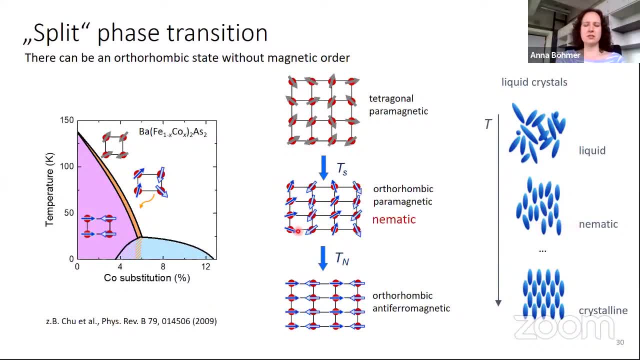 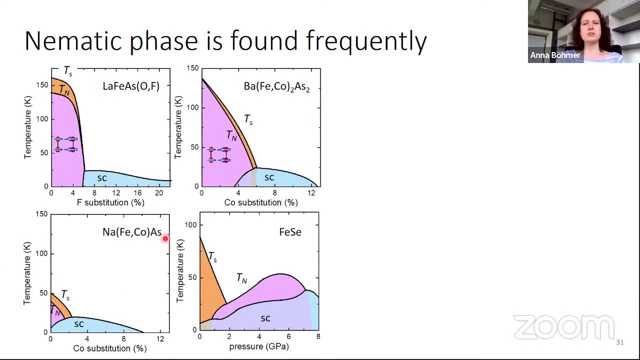 perfect order. That is nematic. That's why we call our state nematic. So in this phase diagram there's an intermediate nematic state. It turns out this is actually frequent, this intermediate nematic state. I have different materials here. All the orange ones are dead. 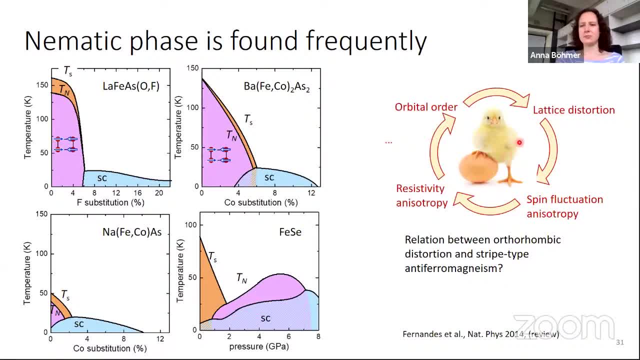 And the question that I've already alluded to is: what comes first, Chicken or egg? Is the magnetism causing the distortion? Is the distortion causing magnetism? Well, we talk about fluctuating magnetism, sort of sort of disordered magnetism here, but really, what comes first has been discussed a lot. 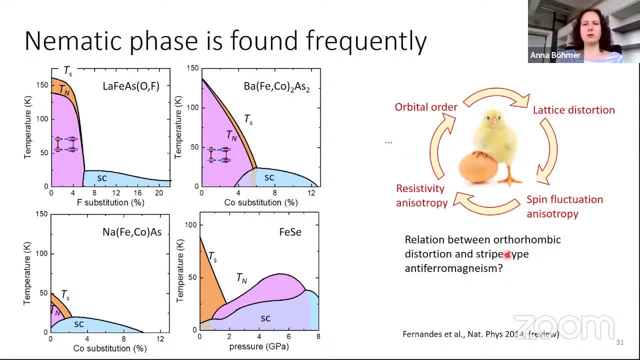 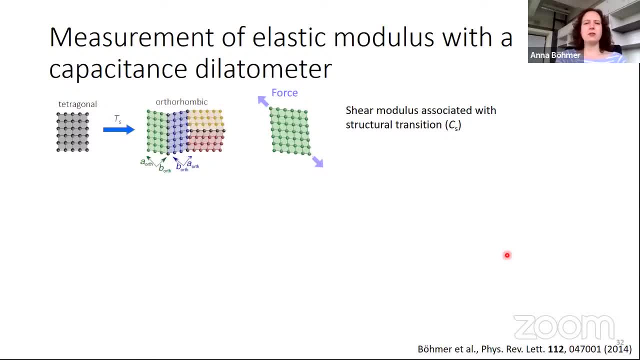 What's the relation? And let me tell you a little bit about what we learned or what we found out. Well, what we used is- it's, I think, cool- a new way to measure an elastic modulus using a capacitance stelatometer. What we do is: 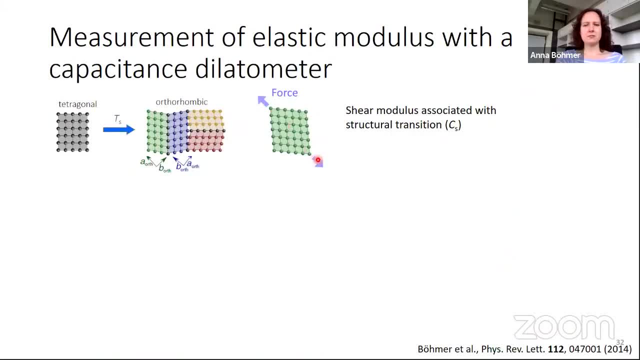 we basically apply a force to our crystal, Sorry. So we go back and force between here and we measure how much force we need for dilating the crystal by a certain amount. That's called shear modulus and the technique is actually old. It's a three-point bending. 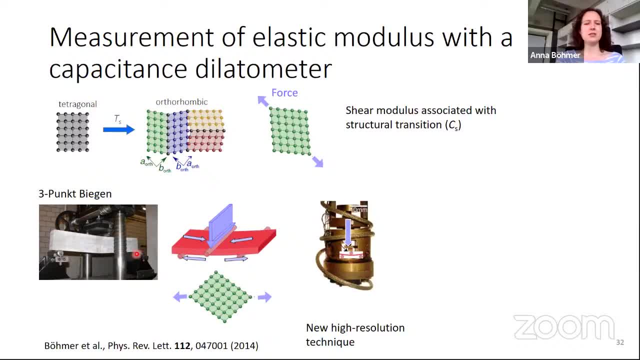 and that's been used in engineering forever. When you want to build a bridge, you want to test your material. that's what you do. But we do it in our dilatometer. So we apply a little bit of force and we measure length change how much, how much this bends. 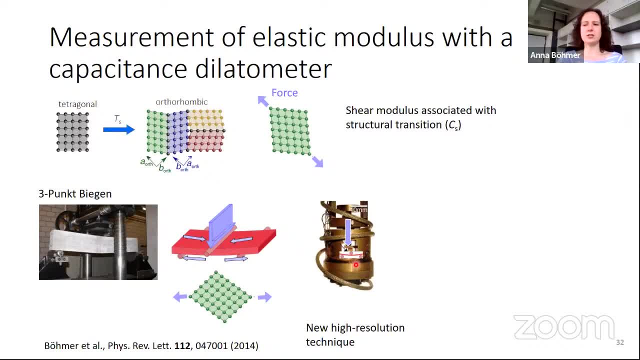 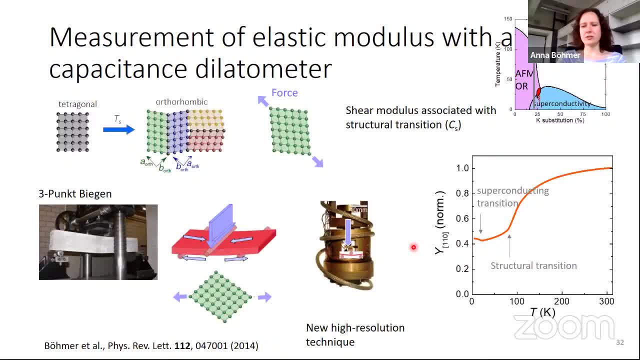 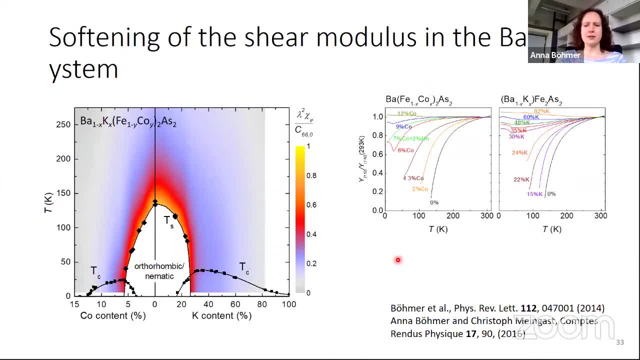 little bit less on the superconducting transition. So there's the competition again, this antagonistic behavior. We did that all over the phase diagram So you can make fancy cameras, plots out of this data. how much material is soft? The quantity you can get from this is: 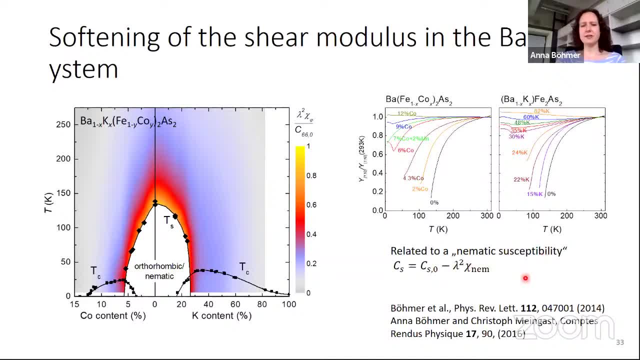 termed nematic susceptibility. So nematic was our distorted state, the strange orange one that we don't quite understand. yet Susceptibility means how susceptible is the material to get into that state? how easy can you drive the system into this state? 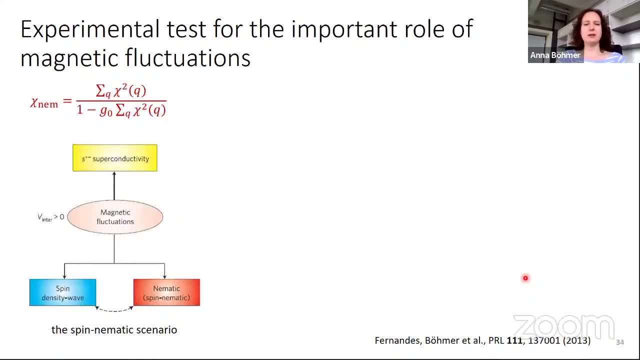 There has been theories on this and here's where I really went to. I really needed the theory and I asked the men and they actually came to us with their ideas. They say: if we can calculate that nematic susceptibility, let's see if you can measure it and we'll compare. 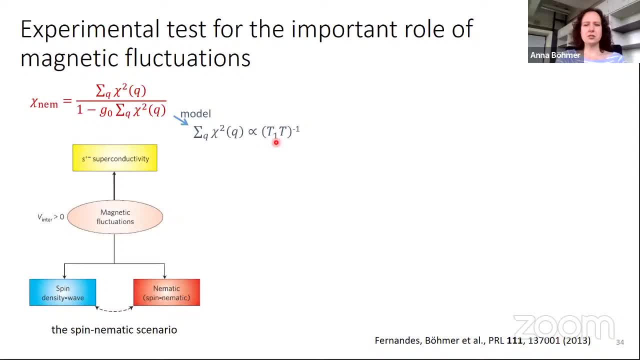 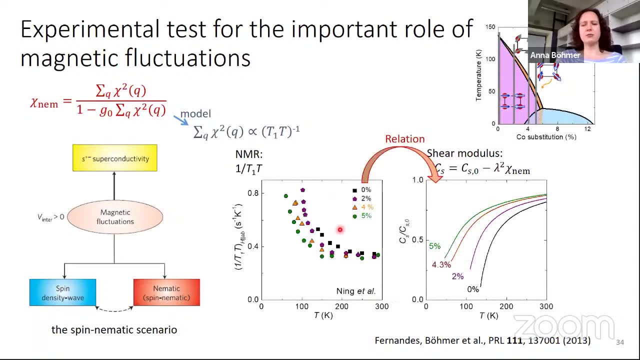 So they calculate. it looks like this: they put a model in it and then they say: here's a quantity you can measure. it's called t1, t spin lattice relaxation rate. The point is it can really be measured. On the other hand, this left hand side I can measure as well. That was my 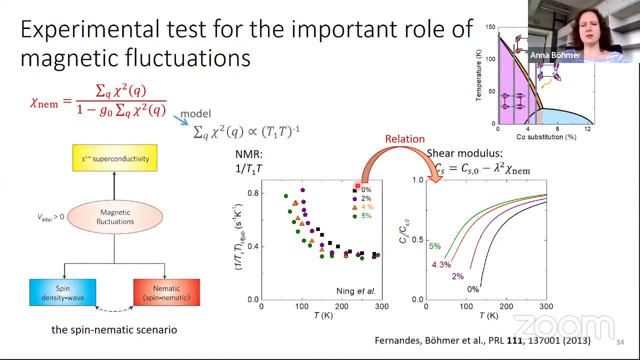 shear modulus. that was my three point bending experiment. The theorist can tell me that there should be a relation between these two And what we do is we test this relation and we scale one data on the other and we find this works, So that theory that starts with a magnetic fluctuations. 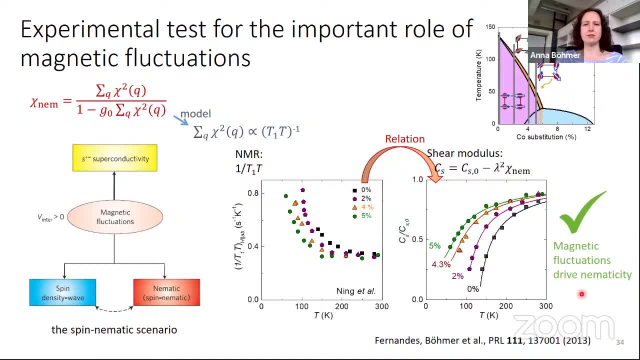 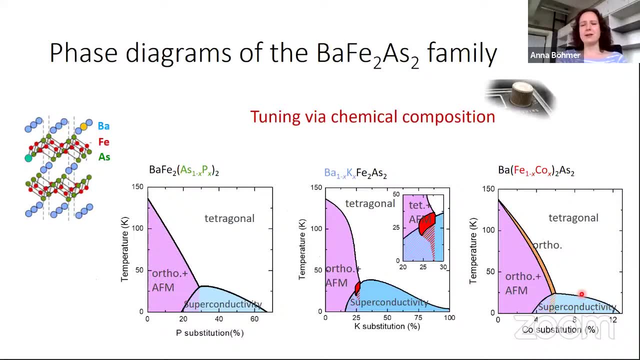 drive nematicity works can explain this data and we found evidence for that And we're quite proud. So let's go back summarize a bit. We've like summaries in terms of phase diagrams. We've seen this one phase diagram with an structural distorted anti-ferromagnetic 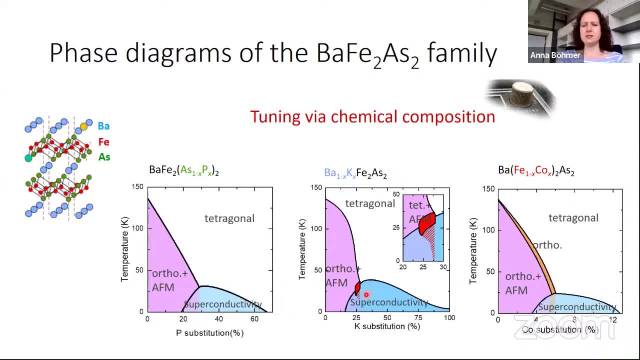 striped type phase and super connectivity. We've seen this intermediate phase where my distortion suddenly disappeared, this little pocket, And we've seen this strip of a strange nematic phase that is sort of in between these two. And now it's time to do. 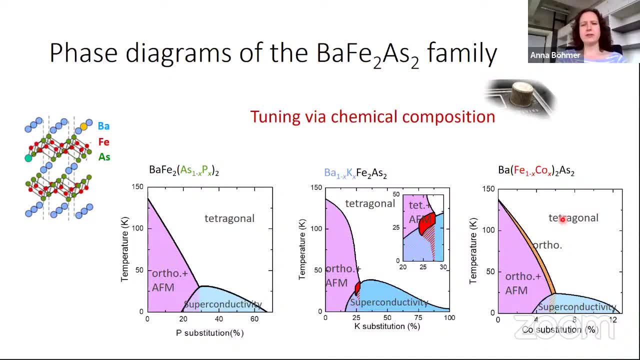 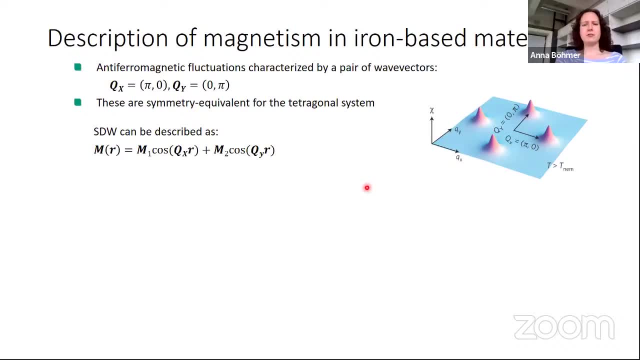 some systematics. So let me try to explain this, because I think it tells us some cool features about how magnetism can be. We go to theory again. maybe a few of you are theorists, I don't know. What we want to do is describe magnetic order. 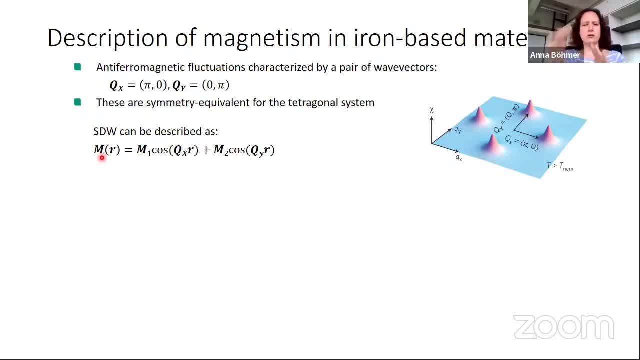 and how these spins are arranged. And when we take a function with this m, it just means what is the magnetic moment? at the position r? We have two m, we have the tutes, two order parameters and two wave vectors, qx and qy. 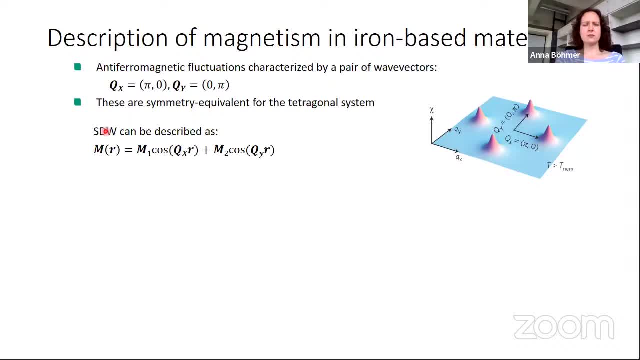 They are in the lattice And that's more generally how to describe an anti-ferromagnetic state in our case. And it turns out you cannot have any values for these two order parameters. You can have. they have relations. There's three options. 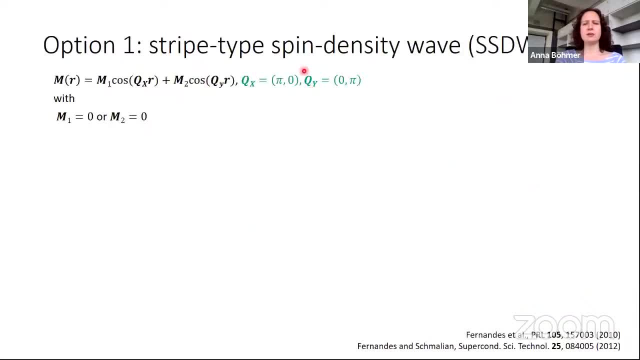 And let's go through these three options quickly. The first one is our stripes spin density wave that you can see here. It is when it's found when one of these order parameters is zero. So then you have just one of these cosine functions. 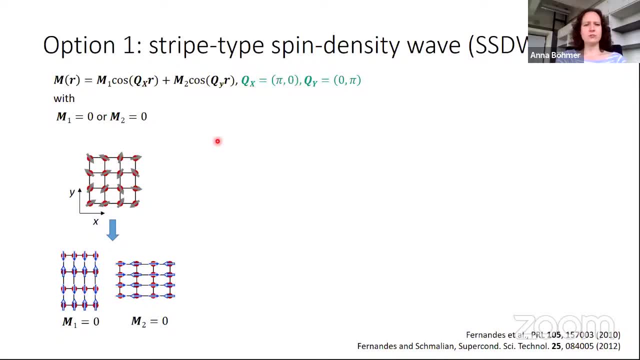 So cosine along one direction. the other direction is zero. So ferromagnetic in one direction, anti-ferromagnetic in the other, And depending on which one of these amplitudes is zero, you find the left sort of stripe or the right one. 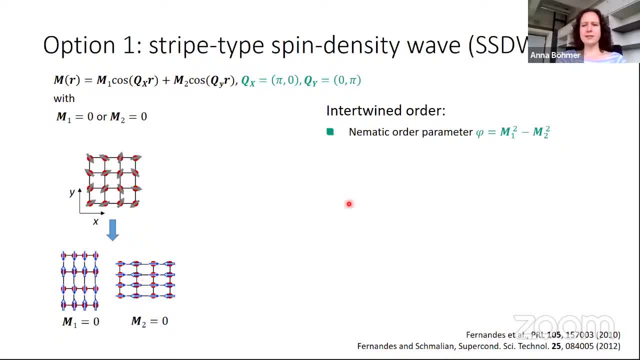 So there's a choice here. I have either this one or that one, And that's exactly my. the magnetic moment, The magnetic order parameter: You can mathematically this is one or minus one if, depending on whether you chose the left. 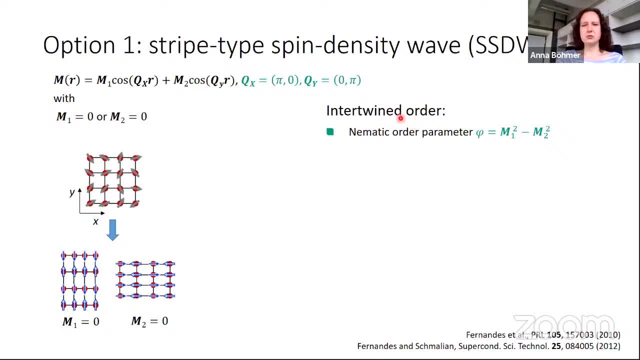 or the right option And the name we gave for this. it's a new order, It's a new choice, It's an intertwined order of our mechanism, Something higher order, something new, something immersion, And we already talked about the magnetic susceptibility. 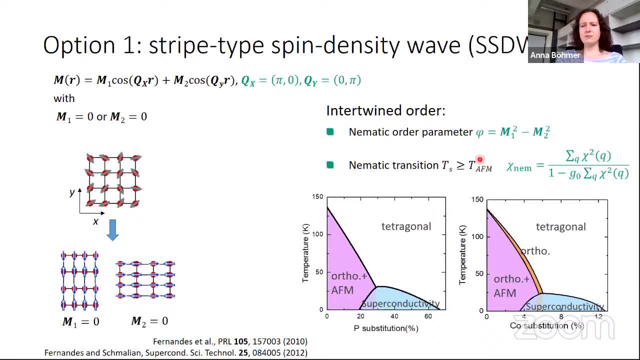 The point is- and it comes from this theory- is we can find this nematic order parameter that has to do with the magnetism, even if the magnetism itself is still absent, Or, in terms of transition temperatures, find the nematic and structural transition. 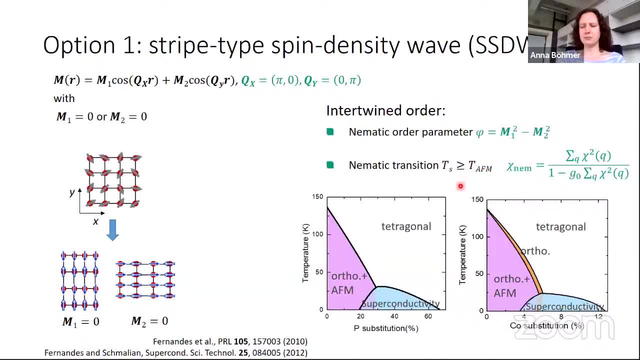 at a higher temperature, or we can find it at a higher temperature than the magnetic one And we experimentalists already knew that. we saw it before. We have it in this phase diagram here: Find the nematic before the magnetic. But there is another option. 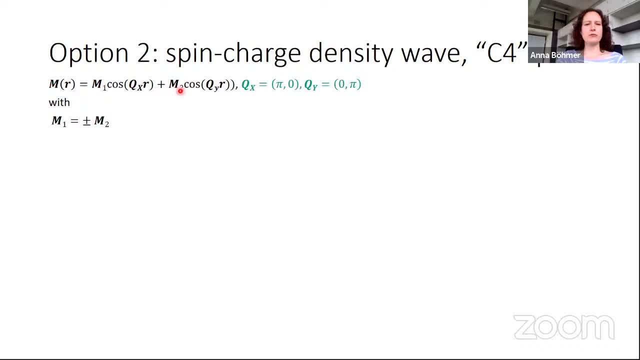 And that one would be: both are of same size and is a parallel or anti-parallel. What would that look like? And you can really make a cartoon trying to add these two terms side per side. So this side, that will just double. 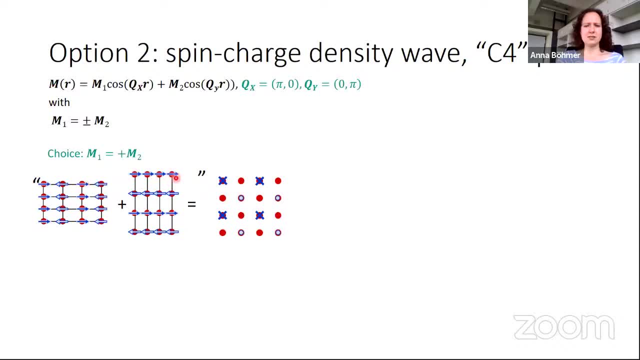 the next side will cancel, the next side will double, the next side will cancel, And, it turns out, the orientation of the moment turns. instead of being in the plane, they come out of the plane. so here my little symbols mean in and out. 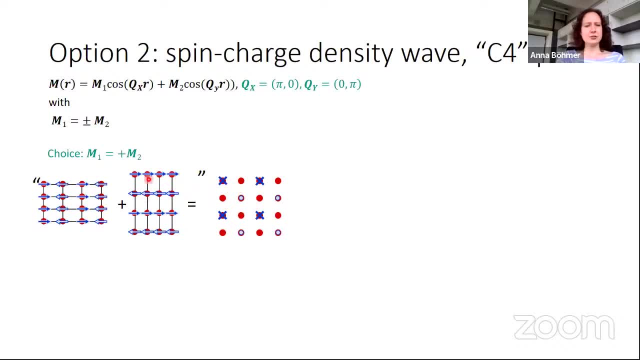 out of the screen or into the screen, And that's the choice. the two are parallel. There's a choice: the two are anti-parallel. And then we find this sort of pattern. You can really edit now: now these two add and the first one would cancel. 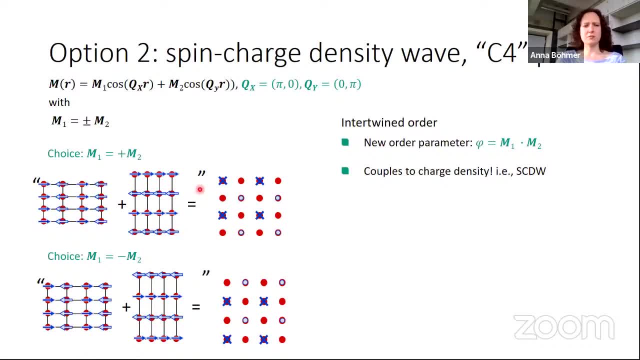 for example. So there is a new intertwined parameter, a new choice. The choice is: are these two parallel, same sign, or anti-parallel, opposite signs, And you can define a new order parameter. And it turns out this is really difficult to measure. 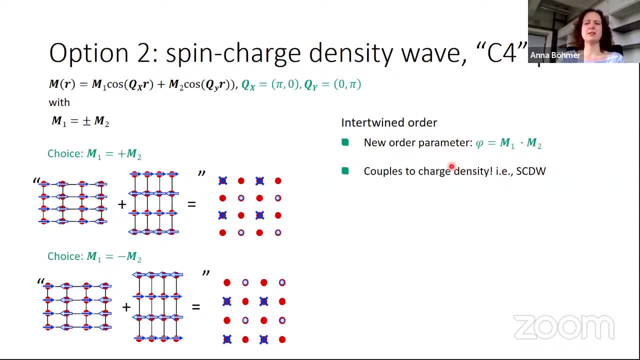 It couples. what it couples to is local charge density and we haven't seen that yet And that is really the phase that was found in the little pocket here. That is has been well, that has been measured using neutron scattering And it was a real one, not only neutron scattering. 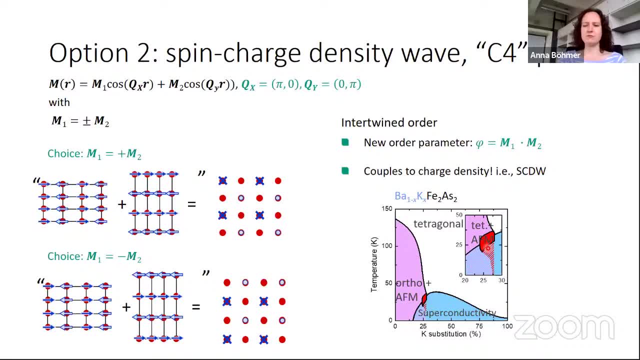 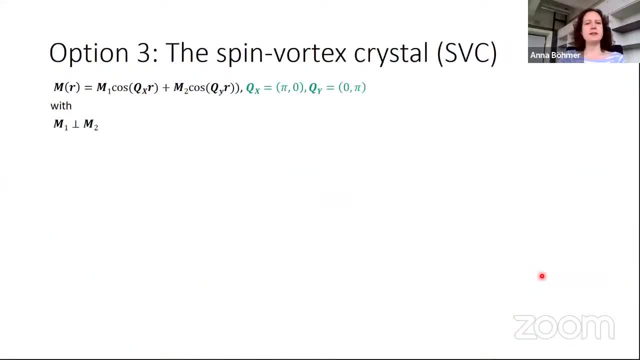 a couple of different magnetic probes, It has been found And this is the face that was found here. So we solved the puzzle. What is this little pocket face here? It's option two And there was an option three. Option three is if the two order parameters 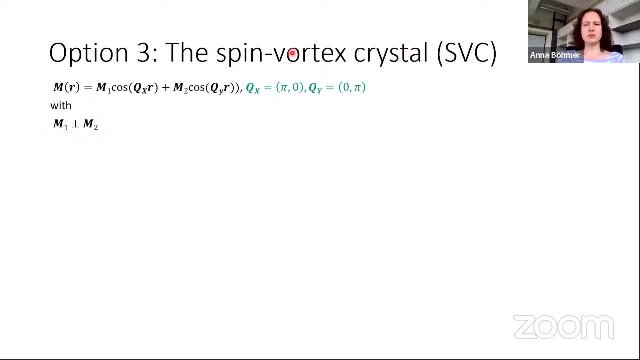 are perpendicular to each other And was termed spin vortex crystal. quite a fancy name. Turns out it's a confusing name because they're also superconducting vortices. But this is a magnetic vortex. What does it look like? So I have the two choices. 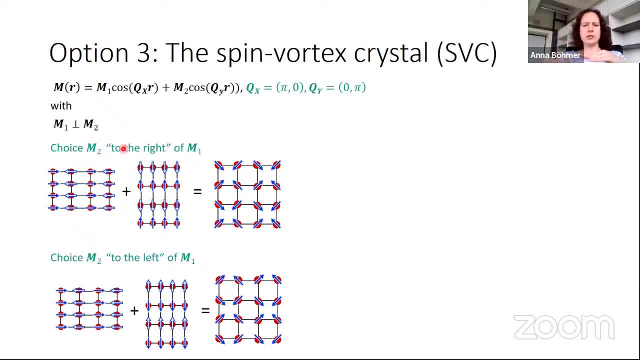 Two choices already drawn out here. Things are perpendicular to each other. One can, but they have directions. One can be to the right or to the left of the other. We get this sort of pattern. You can also add them, So to the right and to the bottom. together gives this corner. 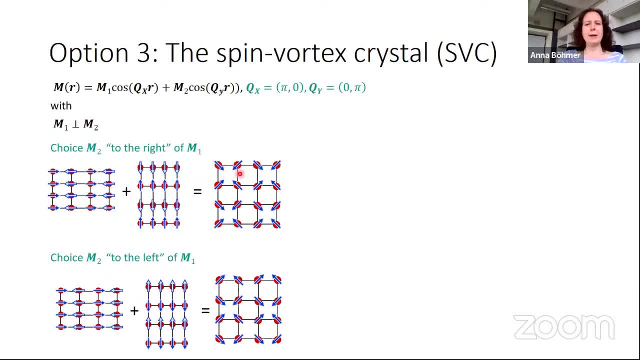 To the left and to the bottom gives into the other corner. If you go around one of these placards, there's sort of a rotation of the magnetic moment. That's what's. there comes this magnetic vortex Where this name comes from. 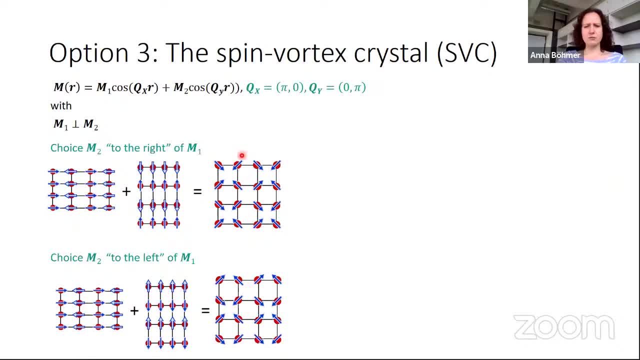 We have again two choices: The patterns. it's a bit hard to distinguish, It's a shift, sort of a phase shift, these two choices. We gave another name to this order: hedgehog, because it's some all out, all in structure. 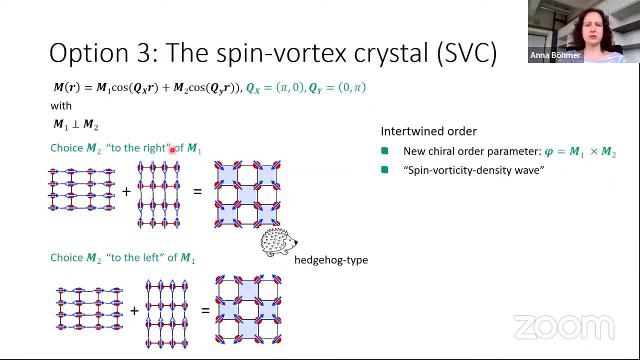 And our intertwined order. our new order parameter is a choice, well, to the right or to the left, And that's the cross product, the vector product of these two order parameters. It got a name. The question was: can we find it? 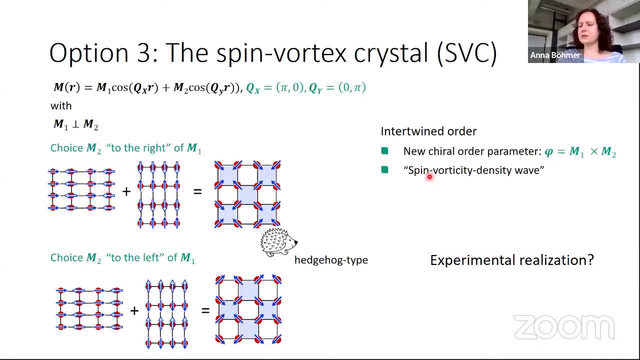 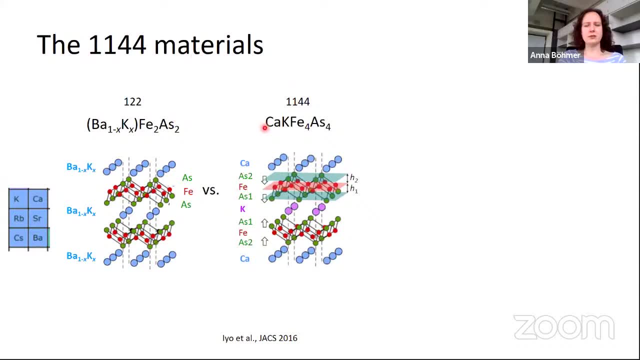 Can we do it experimentally? And I will cut this a little bit short. We did find it in a new material of 1144 material. So just for chemists, maybe among you, that's structure where we have our familiar iron layers. 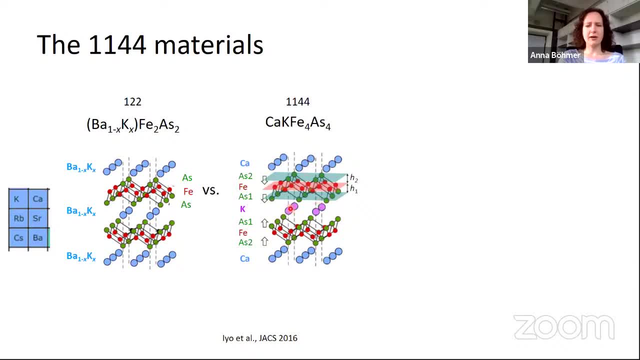 That's where the magnetic moments lie. We have arsenic around, Then we have, in this case, potassium and calcium alternating. So it's not an alloy, It's a 1144, a quaternary compound. It's a superconducting compound. 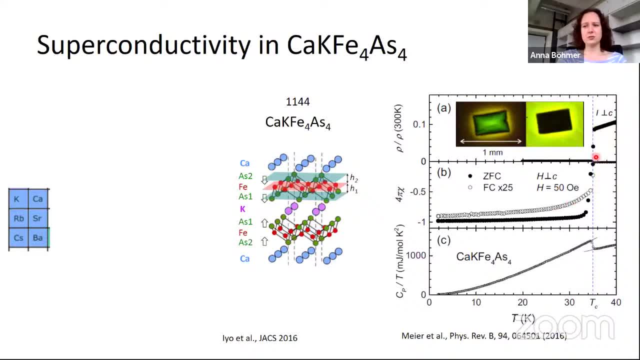 That was seen quickly. You can just measure resistance again. So here's the resistance curve, Here's the diamagnetism, Here's the specific heat jump that I mentioned. It's a nice superconductor. The question was: can we get it magnetic? 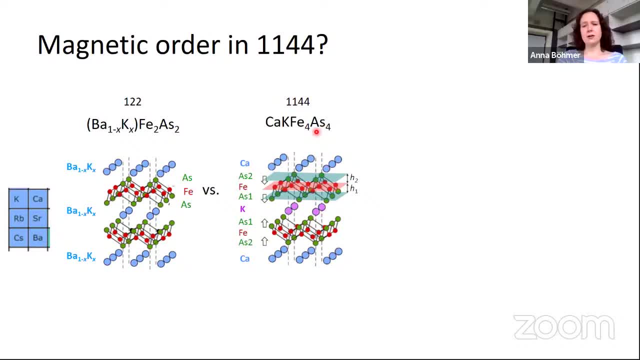 Can we get this compound to be magnetic? by? well, the same procedure we've used Before, chemical substitution, the same things we did before here, And it turns out, if we think about that, a promising way would be to substitute the iron. 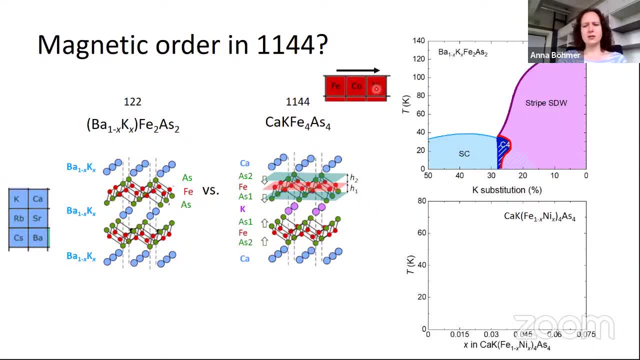 with cobalt or nickel. There's a reason for that, but let's just see what this gives. So now I have an empty phase diagram here: temperature and nickel content in my calcium, potassium, iron for arsenic, And we measured resistance and we found something. 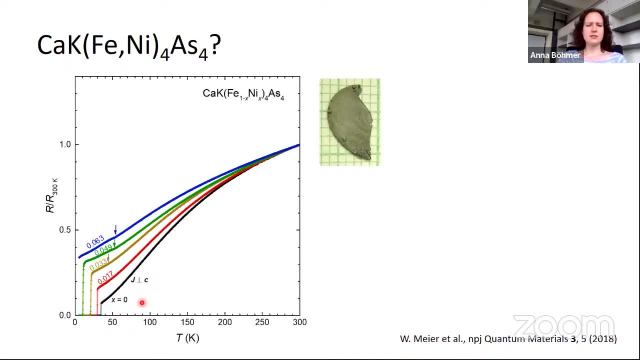 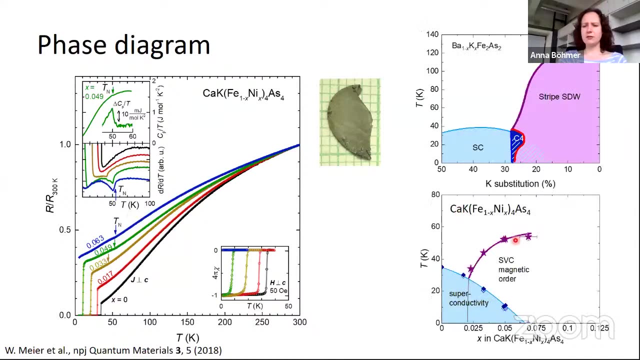 So you've seen the superconductivity, the zero resistance states and you see little kinks here. You take the temperature derivative of the curves and you see a transition. You put all of this together and here's my new phase diagram. We have magnetic order here. 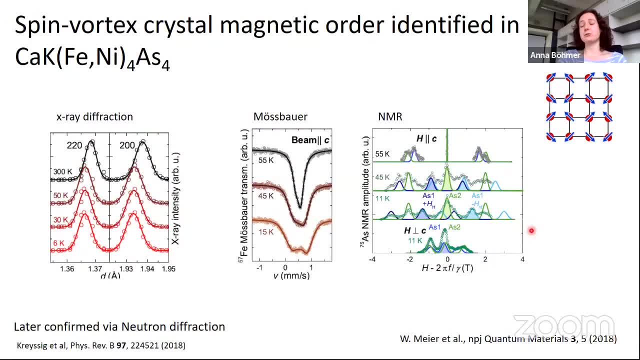 and well then, once you see magnetic order, you want to know what is it? How are the moments aligned? What's the pattern? And we find it's really the hedgehog type spin vortex crystal order, our missing option three, using a couple of different probes- They were all in-house. 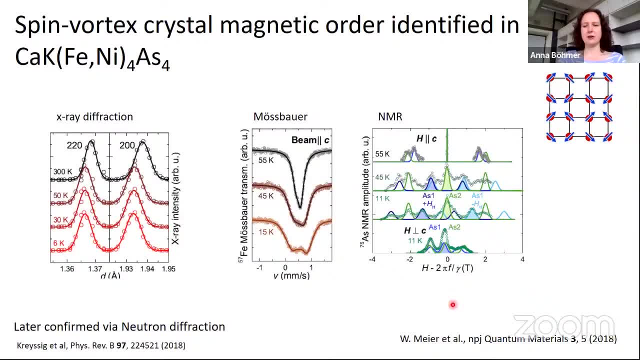 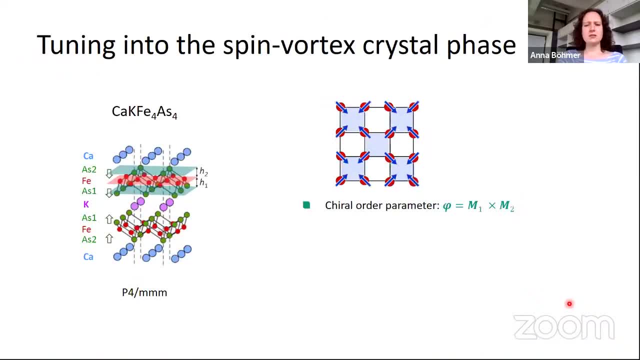 and it's a teamwork. That was a good example of how many groups can work together to solve such a puzzle. There is a reason of why we find exactly this complicated structure and exactly this material, and has to do with my intertwined order, with these two amplitudes, two order parameters. 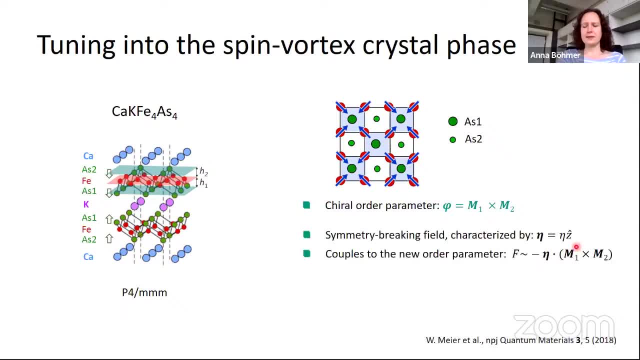 and the vector product Maybe for well, it's a structural reason. it has to do with these alternating layers, say so much. So we understood why likely we got this. We are not sure, but we understand why it's more likely to get this option three, magnetic phase- in this material. 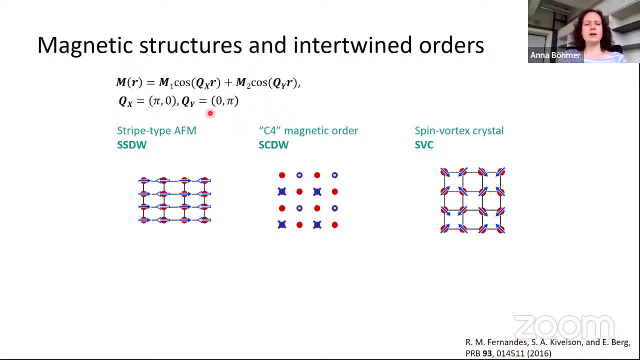 With this I would like to summarize: In these iron-based materials we have complex magnetism can be described in this way- and we find three options, three different patterns coming from the same mechanism, same wave vectors. We find the stripe type with the interesting coupling. 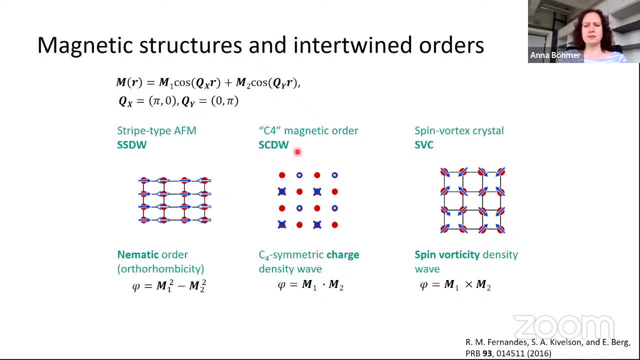 to the structure and dynamicity. We find the spin charge density wave, this alternating one, where moments sometimes cancel, And we found the spin vortex crystal, where moments rotate within the plane Each time there is some new emergent order parameter, which is a concept. 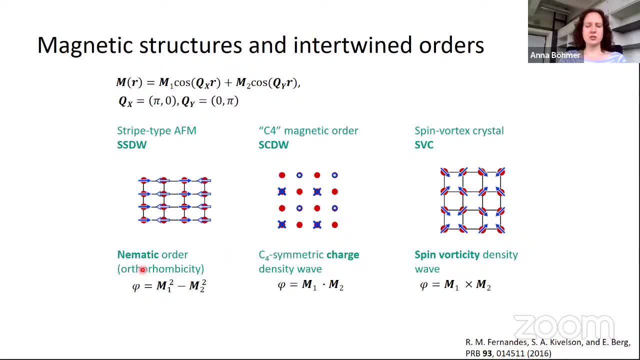 in this sort of physics and which sometimes we can measure easily And sometimes we can't, And this led us to some tuning: Tuning using some forces coupling to this, or tuning using this structure, this alternating layers. Here we couldn't find out how to tune this. 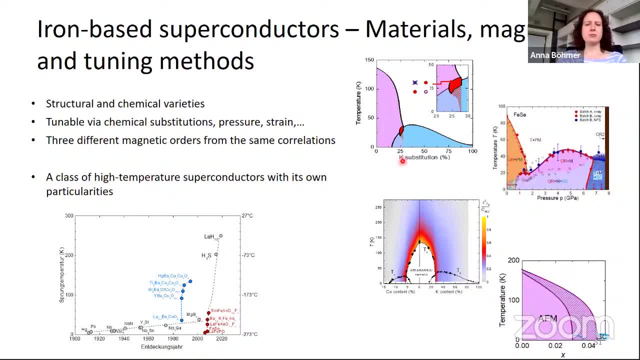 So, finally, on materials, magnetism and tuning methods and iron-based superconductors, We've seen a lot of structural and chemical varieties of the materials that are tunable, that properties can be changed using chemical substitutions, losing pressure, using distortions, using the C over A ratio, as we did with the substrate. 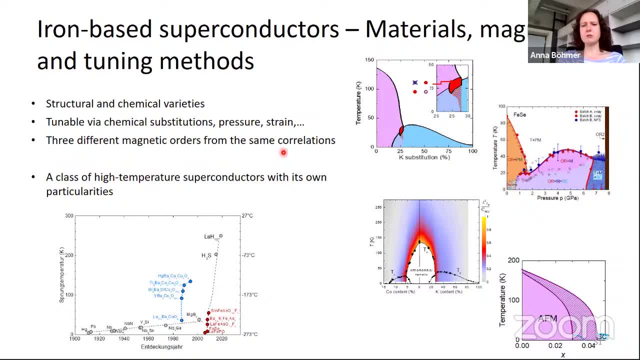 And we've seen three different types of magnetic orders from the same sort of underlying magnetism and with each one an intertwined, much remarking emergent order parameter. So all together, we have here at hand a class of high-temperature superconductors. 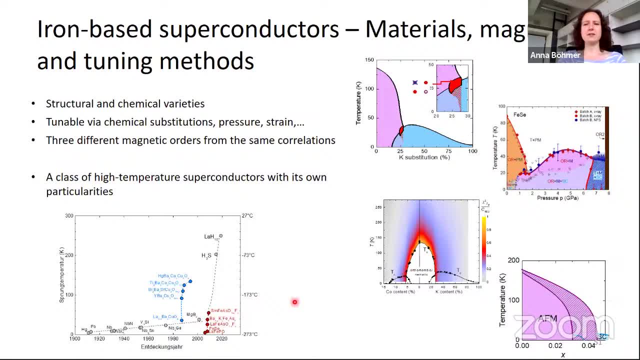 That are tunable, That properties can be changed using chemical substitutions, using pressure, own particularities that are very worthwhile exploring. Thank you very much. So thank you very much, Anna, for this wonderful talk. So now, please, if you have questions, write them in the chat or raise your hand. 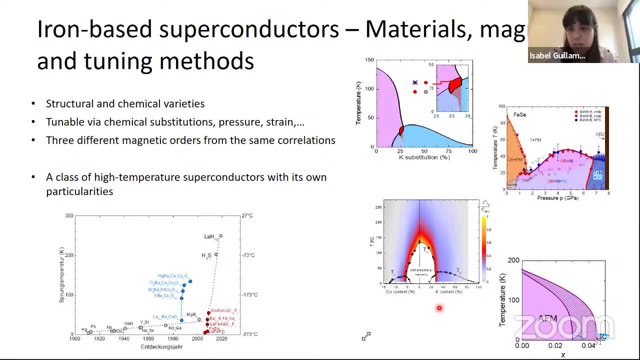 I cannot see questions. Maybe I can start making some questions. So in this potassium-doped barium-1,2,2 system you have discovered this intermediate phase here in red, So maybe I missed it, but is this phase superconducting? 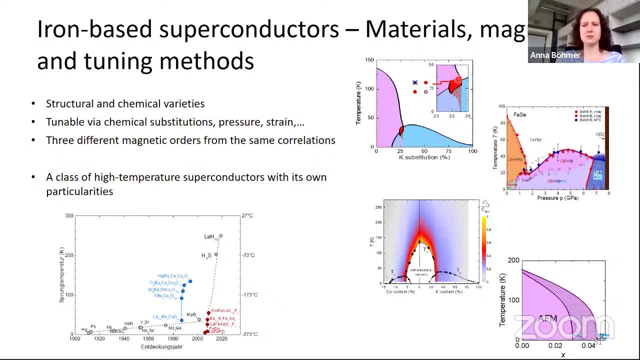 Sometimes It is a magnetic phase. It's this magnetic pattern and it sometimes can be superconducting, So it's the same as Okay, It's an aspect I didn't really touch upon a little bit. I said that the oseromic distortion is decreased in the superconducting state, but it's still there. 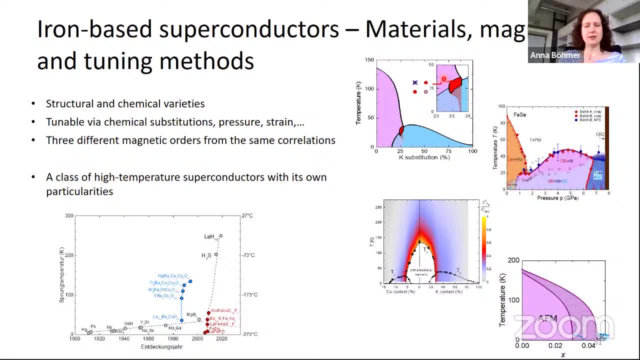 So there's a superconductor that's oseromic and magnetic and there's also a superconductor with this sort of other magnetic order and superconductivity, And maybe, Maybe, one thing you can learn. It's a little small here, but something you can learn from. 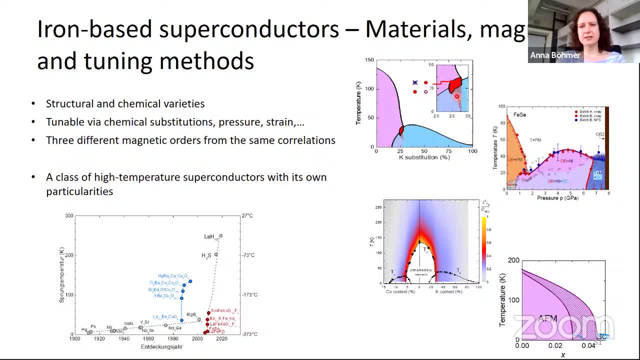 these lines in the phase diagram is this line. It goes like this: So it means that the superconductor still would rather prefer the stripe magnetic order than the tetragonal, the spin charge density wave order. So it prefers the pink to the red. You can see that because the 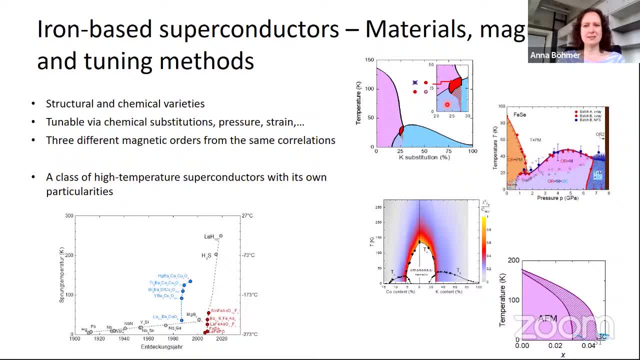 red region shrinks inside the superconducting state. Okay, So there's different degrees of competition between these all these phases. Okay, so then, because you have described different kinds of magnetic orders: the striped antipyramidism, which is the more, the most common, and also this: 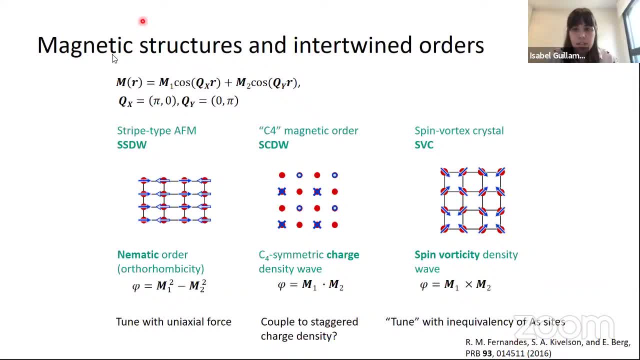 spin crystal, spin vortex crystal, antipyramidism. so which do you think is competing more effectively with superconductivity? Oh, that's a good question. So it's a little hard to answer that using my 1144 material, the one that I talked about, because that one does not have stripe. 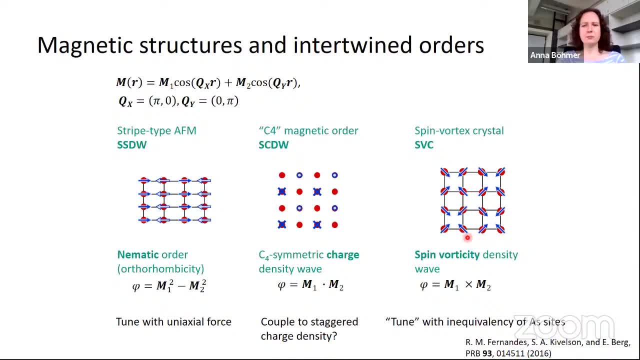 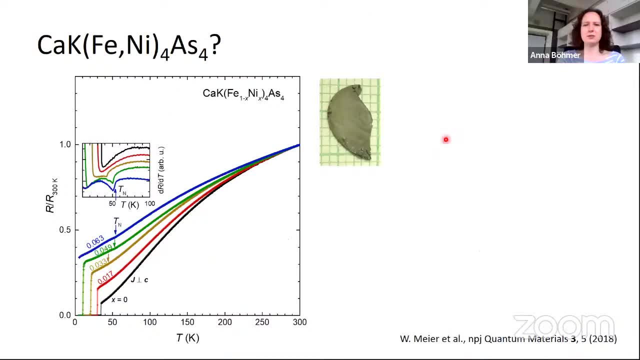 To answer that you need a material that has ideally, all three of them and superconductivity, and luckily we have one of these. So I skipped over that because I felt it's maybe a bit complex. Let me see I need to go back. 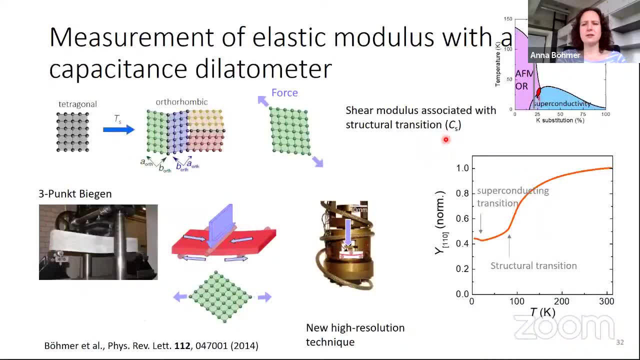 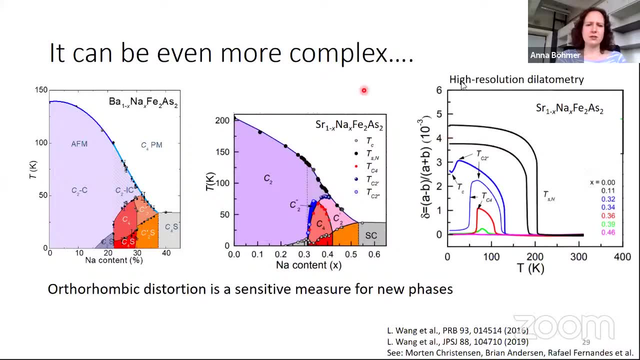 Screen sharing, Because it's here. So there is this one material, the sodium. Let's go here. So here I think you have all three phases. You have the striped phase here, you have the one with the moments in and out and partially cancelling my option two here, And this very 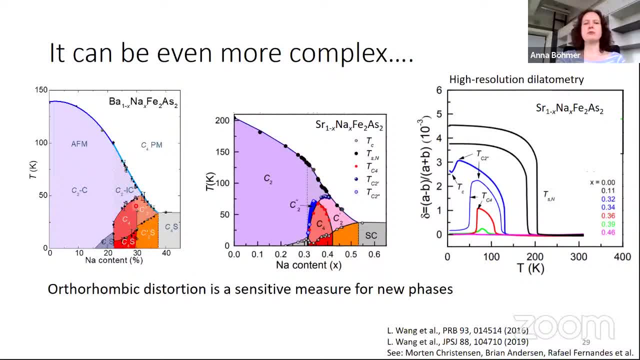 recently was found evidence that it's a spin vortex crystal. Okay, And now you can look at the superconductivity. that's the phase line down here And I think I think what you can learn is that the C4 phase is the worst. So the option two is the worst. 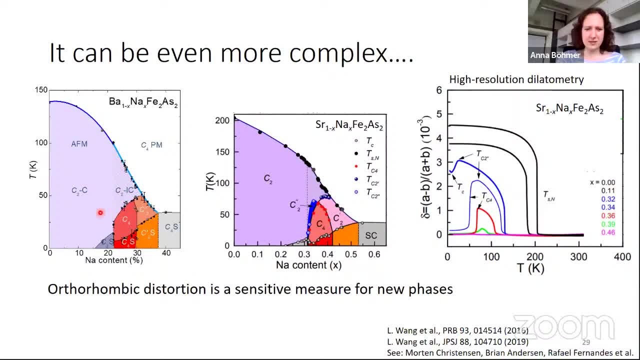 The next worst is the spin vortex crystal And the best is still the striped phase. Okay, And in this work it was related to entropy changes and how much density of states is removed. Maybe you can look it up. There's a reference. 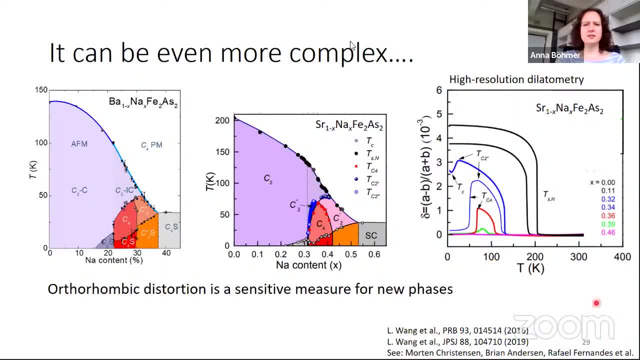 down here, Okay. So yeah, this is. this is very, very impressive work and very interesting, complex material. So many phases. I think there's a lot to be done, still Also quite intimidating. There's a lot to be done there. 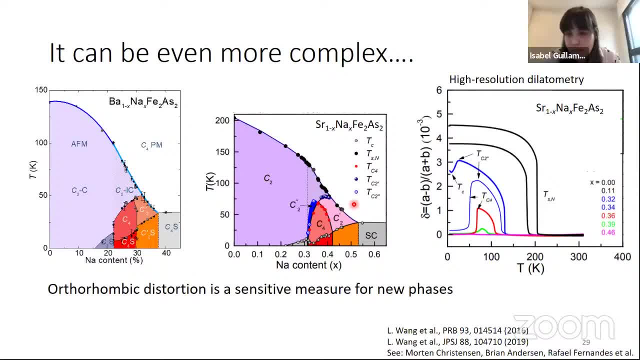 Thank you. Well, there are two questions in the chat. The first one is from Lenovo. Maybe, Lenovo, you can unmute yourself, and or let me try to unmute So you can ask the question yourself. I didn't find out how to read the chat. 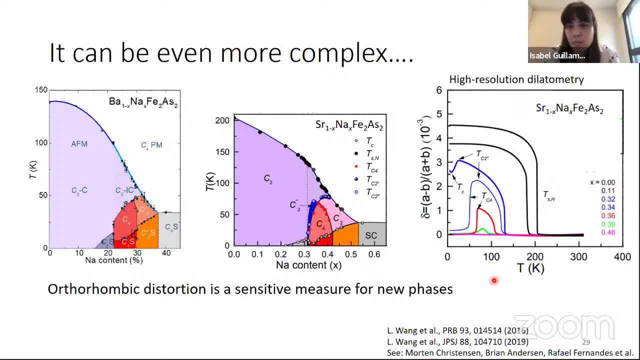 It can be. the question Seems not working, So Lenovo asks: are you consider vacancies in 2D materials as a distortion? Vacancies in 2D materials, Well, there's certainly a strain field associated to them, So a local distortion- When I say distortion here, I mean an ordered one really Like. 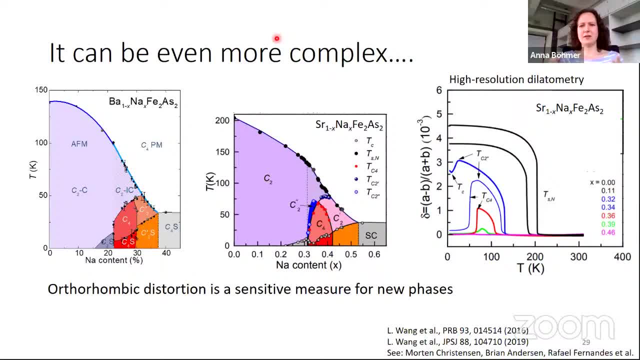 the whole system is distorted in the same way, So I would: it's it's. I don't think it's the same thing here. When I say distortion, it means my whole material starts in the same way. If I have a vacancy that's not ordered. that's inhomogeneous. 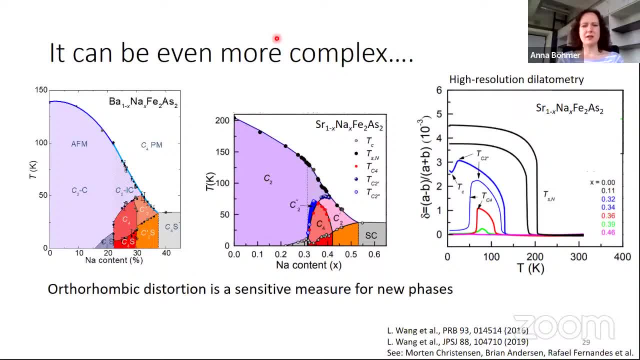 strain. inhomogeneous distortion. It's also interesting, but it's a little bit different, And I think you would not talk about phase transitions there, I think, but I'm not an expert on 2D materials. Okay, So there is another question from Marta. 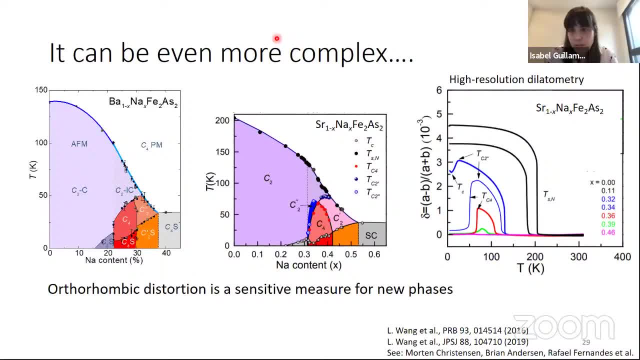 Marta. Yes, Marta, Yes, Maybe you can ask the question yourself. Hi Hi, Very nice talk. My question is: in the STM measurements that you showed before, the ones with the two areas, how do you change the pressure there? Because with the crystal, 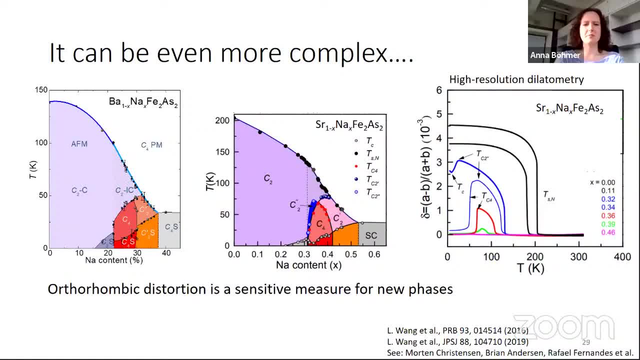 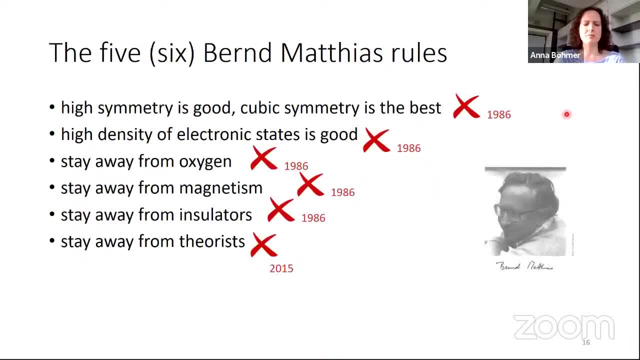 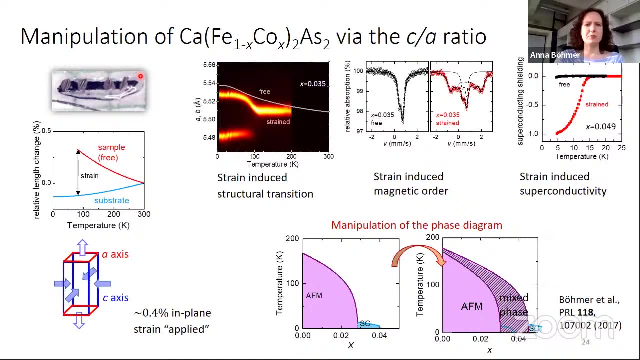 I don't know. Yeah, a good question. You can't. Let me see if I can get that. No, Yeah, There, We have to take the pressure we have we got. So what we have is a substrate and a sample, And the amount of pressure is really given by the mismatch and thermal expansion, The 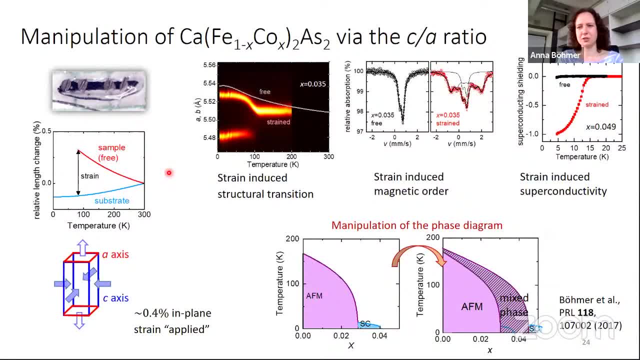 sample wants to expand, it can't. it has to follow the substrate And that's the amount of pressure we have. What you can do- but we didn't- is choose different substrates. So you have a few discrete values you could look at. 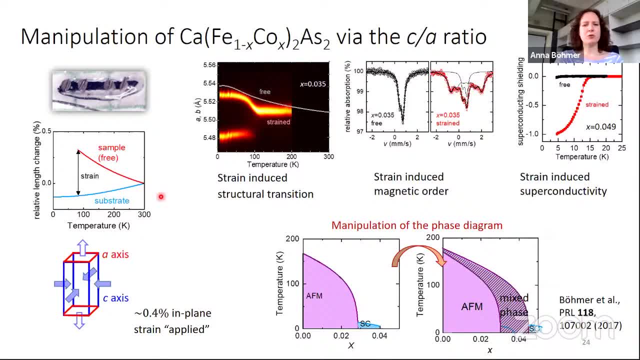 Yes, Um, but we have not explored that systematically, So it's a little bit difficult. And yeah, so. so we have an estimate of how much pressure we have in that one, but we cannot easily change that amount. Okay, Herman has a question. 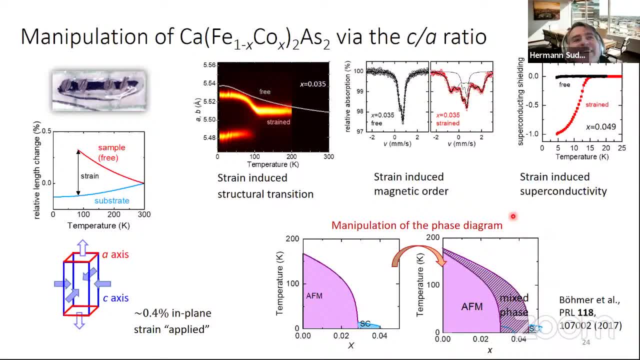 Yeah, Hi, thank you. Thank you very much for the nice talk I have. I have one question in the well, two questions actually. So, when you consider the spin vortex crystal, do you think, I mean you're, you're you present this generic idea of having anti-ferromagnetic order which goes away? 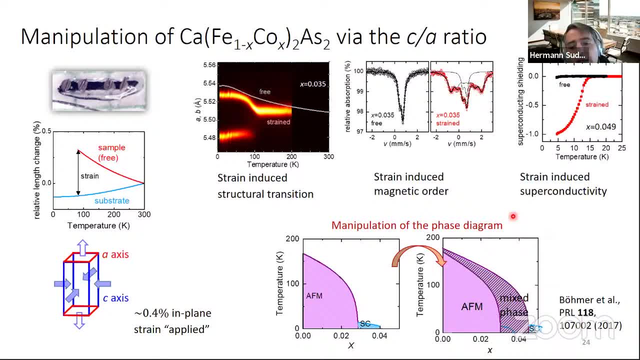 the quantum critical point at some point Now? do you think there is a quantum critical point associated to spin vortex? And and more generically, I mean in most of your measurements? it seems that the quantum critical point is avoided by a lot of faces, right? 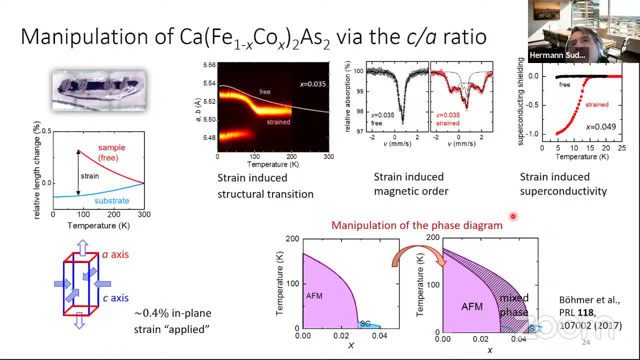 Yes, So what do you? could you comment on that? Yeah, Okay, So the the question of quantum criticality- and that's what I, what I started with, is, of course, um heavily studied here. in the spin vortex crystal material, There is one NMR word that claims to have found evidence for. 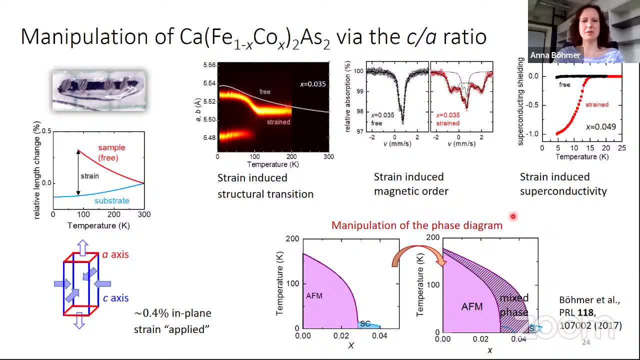 the spin vortex. It's even the title: spin vortex, crystal quantum critical point. They look at magnetic fluctuations in that, But I don't think there's clear-cut evidence for textbook-like behavior there. And there are some materials- the phosphor-stoked barium-122, which I've mentioned. 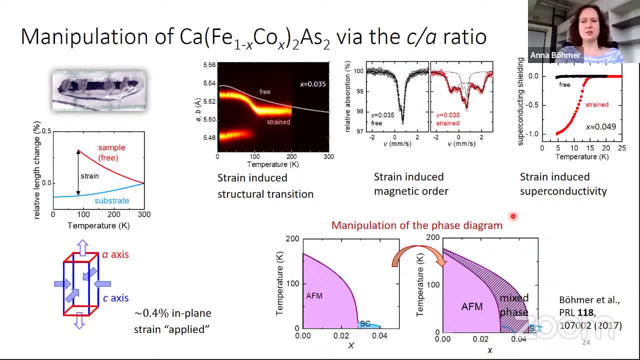 sort of as a simple example where there's more evidence- actually a lot of evidence- for it by now. There was just a symposium yesterday on iron-based using transport measurements, magnetotransport measurements, scaling behavior. They find a sort of scaling behavior that would 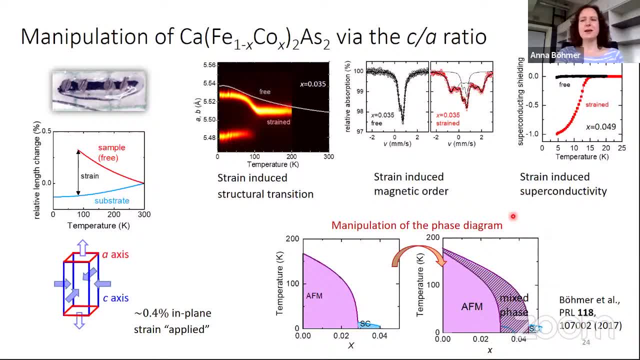 come from these ideas. So, yes, in these materials, at least in some of them, there's evidence for this idea. It's typically done in high magnetic fields to get rid of the superconducting. So we can look at that point, because that's one of these issues. right, We hide that special point. 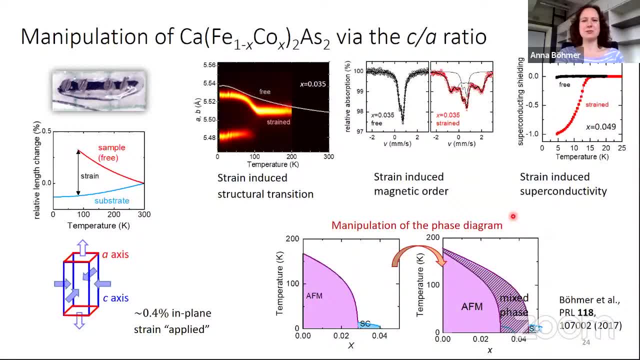 and the superconductivity is so high we can't really look at it. So we need to destroy superconductivity and standard ways to use high fields. In this case, you need 50 Tesla or so. Okay, thank you, Let's see. are there more questions? 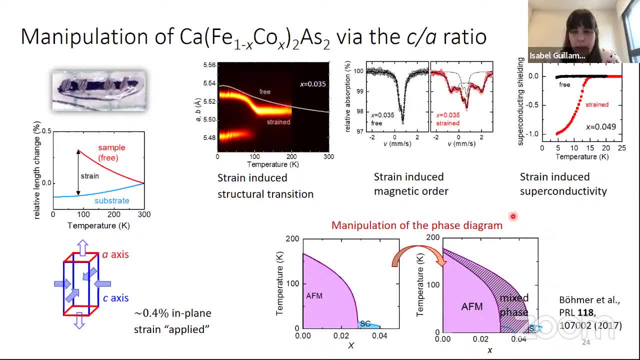 If not, I do have another question, Because you said that the magnetic fluctuation drives nematicity. Is this also true in iron-selenite, Because there the magnetic transition is farther away in the phase diagram? Yeah, that's a good question. That's also an important point. I have not mentioned iron-selenite. 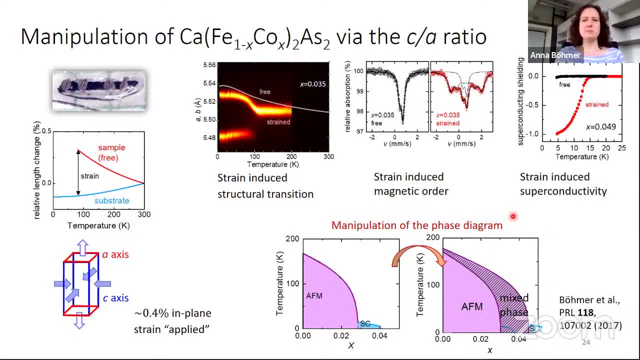 in this talk because I felt this would get us too far. So there's this one material which has a nematic phase- Actually, I have one graph of it, So that's where we picked it up- And no magnetic phase, Maybe. 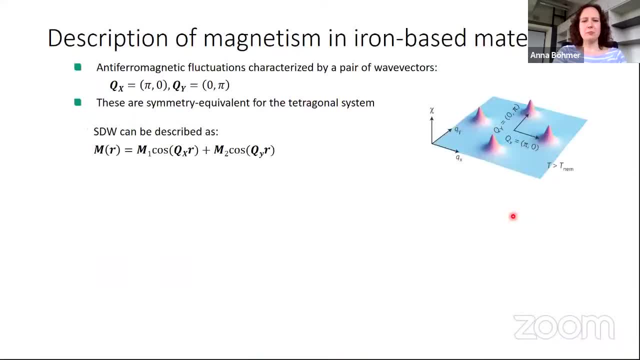 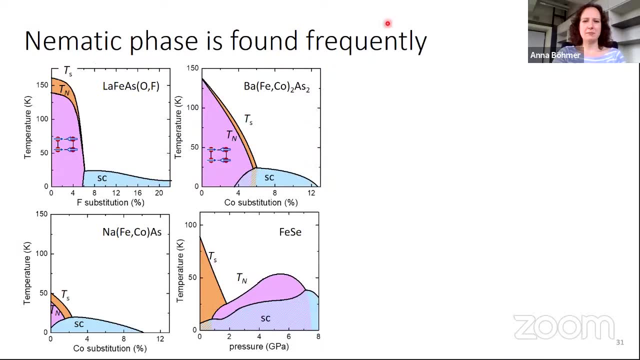 Okay. so my personal opinion is no, But there would be other people in the community that would say yes or yes, maybe. I think it's the bottom right material here. So here we have a nematic phase, Here you have the magnetic phase, And you already. 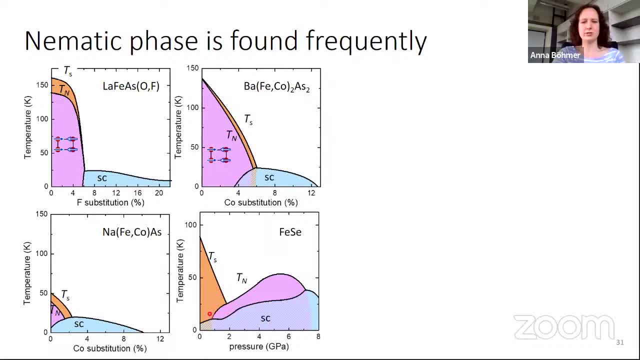 see, the relation is quite different. right, It's not a precursor, It's first, and then gets suppressed, Magnetism comes up. So we studied this a lot And I would say no. I would say there's another reason for the distortion here and a different mechanism for the magnetism here. 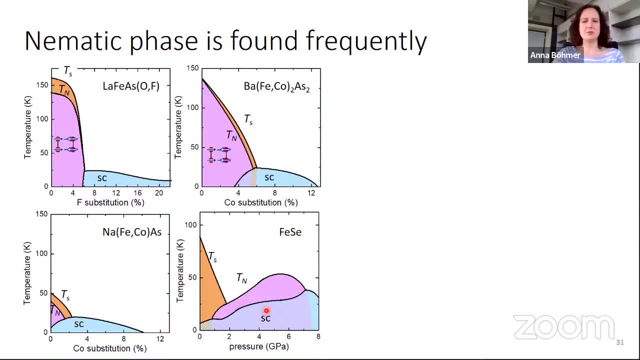 We did finally write it up in a long paper two years ago or so, And that's my opinion, But yeah, I have heard other people saying different things. Okay, Thank you, So I cannot see further questions, So before thanking Ana for